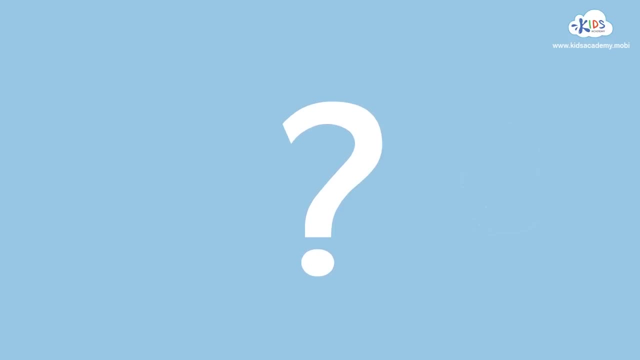 How do we say that there are no snowflakes in the sky? We have a special number that will help us Meet the number zero. Spring is here. Snow and ice melted in the sun. In spring, rain falls from the clouds. 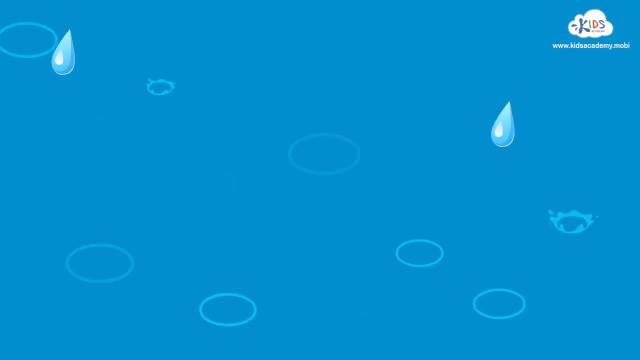 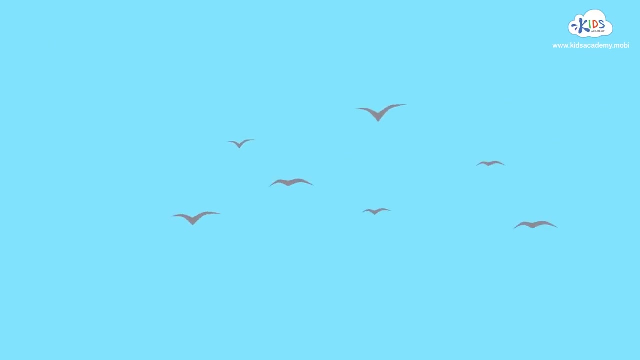 Spring rain goes away soon and tiny raindrops end up in lakes. How do we say there are no raindrops in the sky? The number zero is there to help us. again. Spring is in the air, and so are the twitters and chatter of birds. 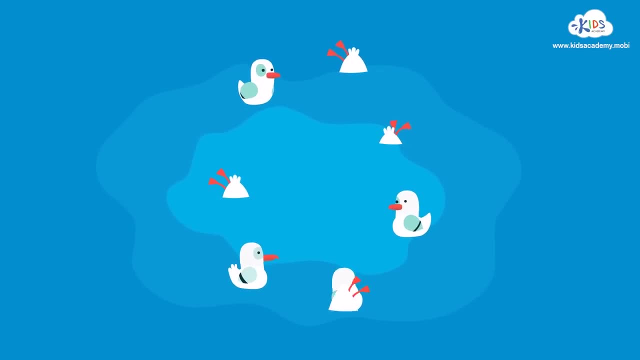 The seagulls are relaxing in the water. The birds flew away. The birds flew away. How do we say there are no birds in the water? The number zero is just what we need, because zero represents absence of a thing. We use all other numbers when we can see some snowflakes, raindrops, birds or other objects. 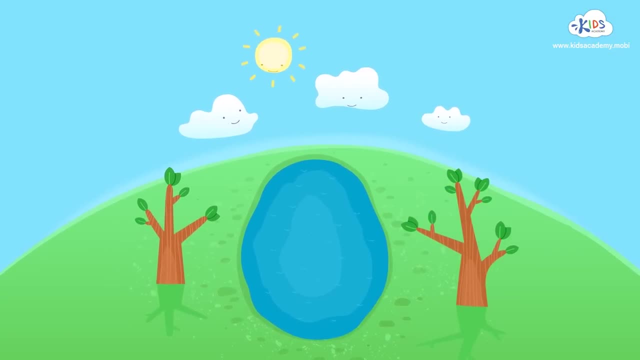 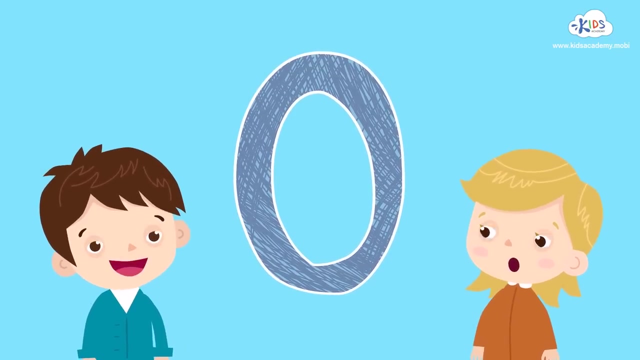 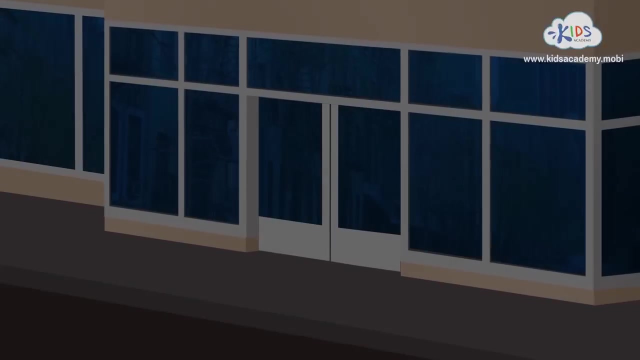 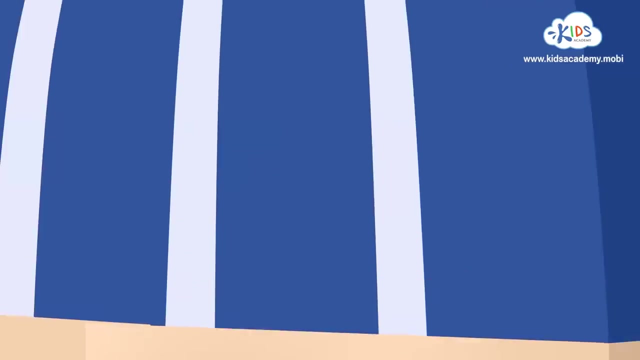 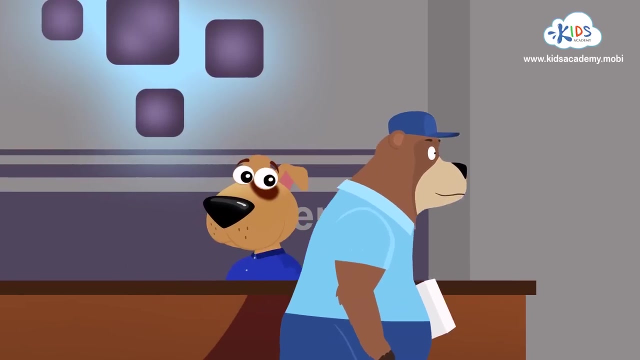 We use zero when there are no objects at all. Hey everybody, it's me, Bernie. I need to deliver this parcel to the 20th floor of this apartment building. If I take that elevator to the top of the building, I can reach the 20th floor really fast. 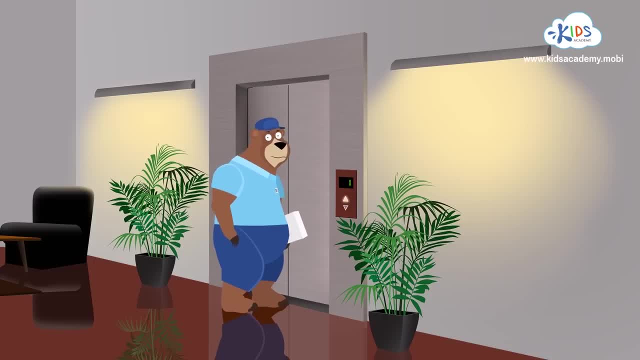 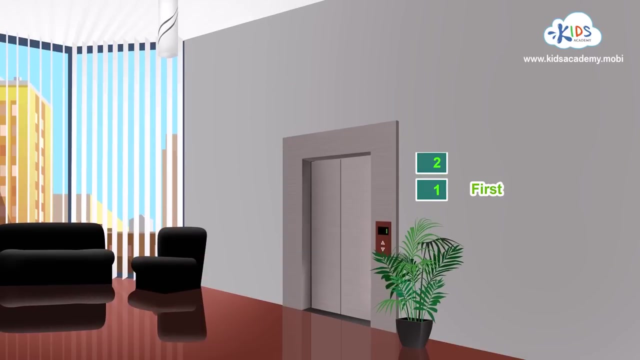 We have to go from the first floor all the way up to the 20th floor. Help me count the floors as I go up so that I won't miss the right one. One: We are on the first floor now. Two: Now we are on the second floor. 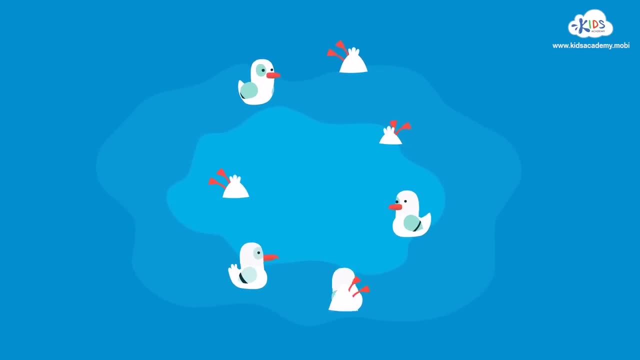 The seagulls are relaxing in the water. The birds flew away. How do we say that there are no birds in the water? The number zero is just what we need, because zero represents absence of a thing. We use all other numbers when we can see some snowflakes, raindrops, birds or other objects. 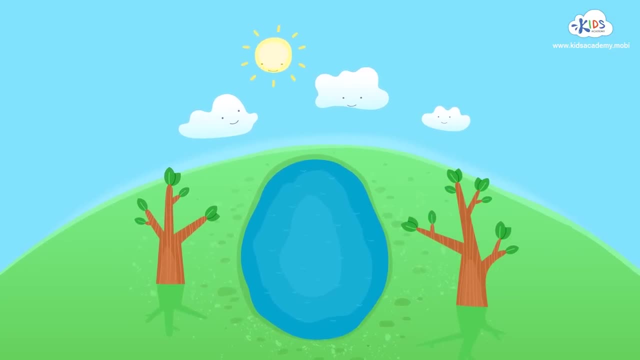 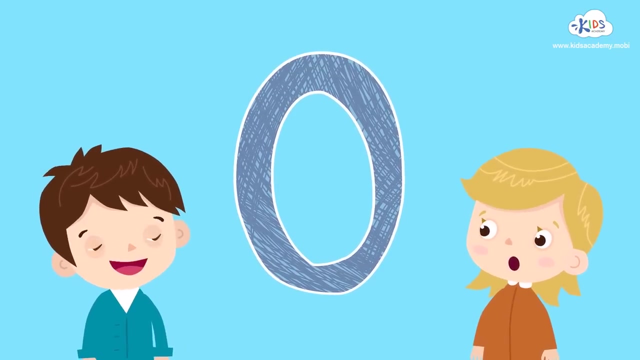 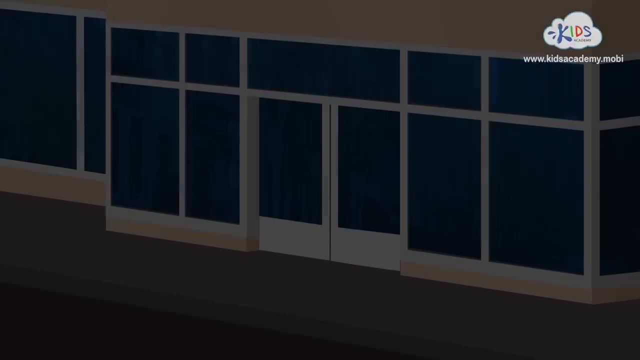 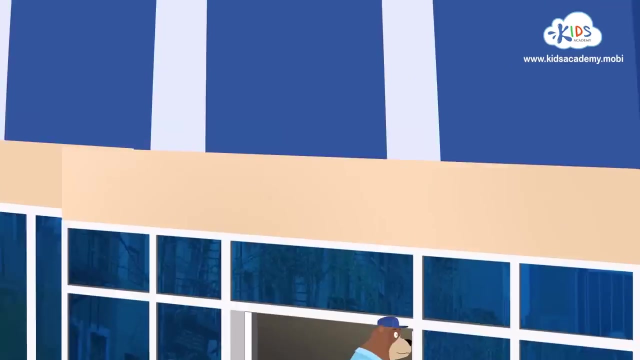 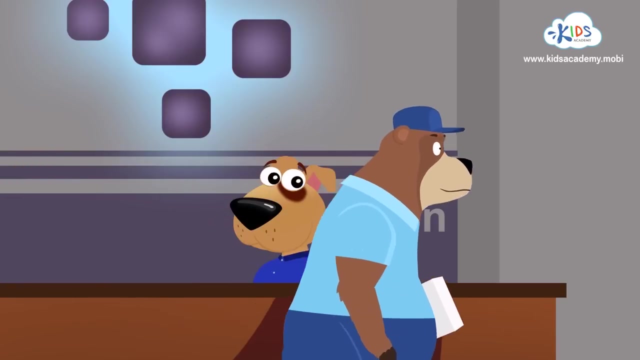 We use zero when there are no objects at all. Where are the birds? Hey everybody, it's me, Bernie. I need to deliver this parcel to the 20th floor of this apartment building. How do we say it's un-brushed? 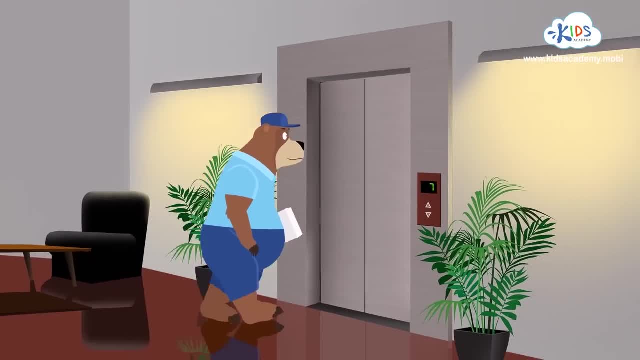 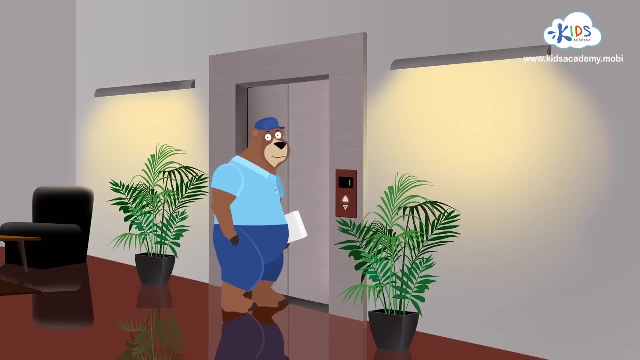 If I take that elevator to the top of the building, how do we say it's un-brushed? I can reach the 20th floor really fast. We have to go from the first floor all the way up to the 20th floor. 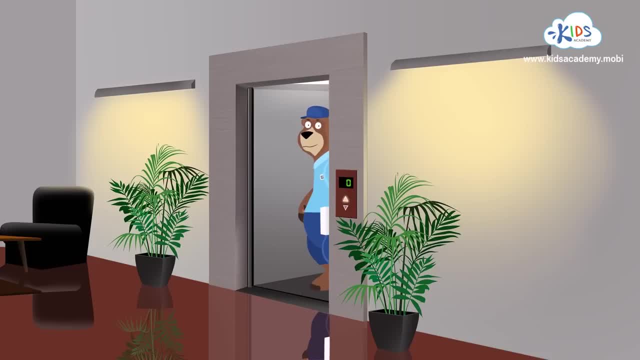 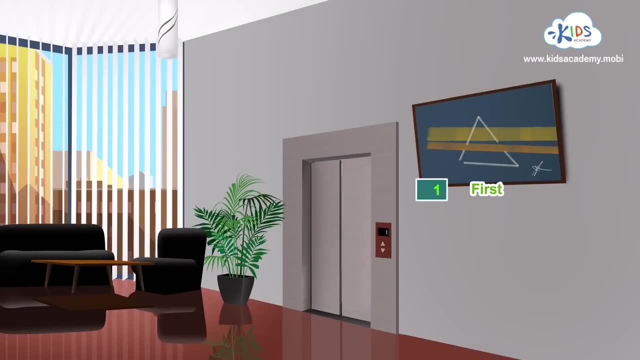 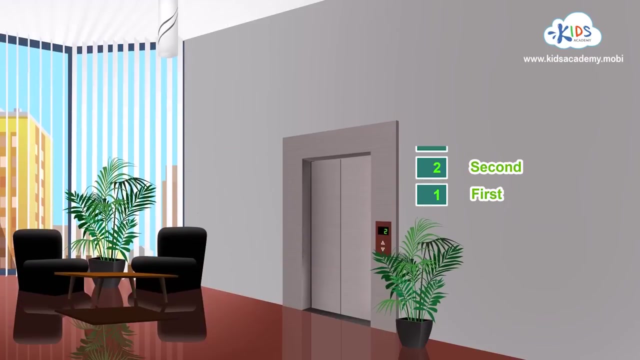 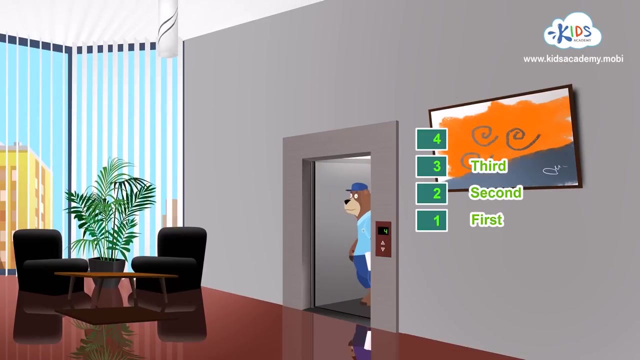 Help me count the floors as I go up so that I won't miss the right one. One: we are on the first floor now. Two: now we are on the second floor. Three: it's the third floor. Four: which floor is that? 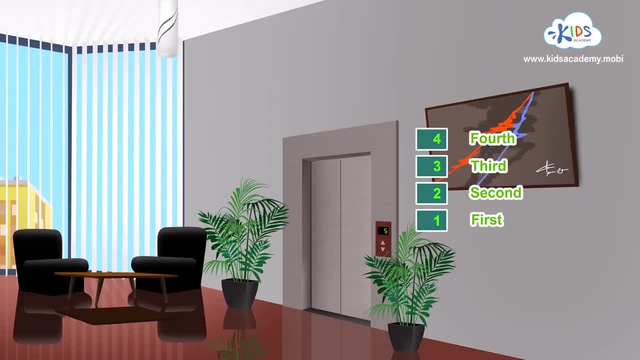 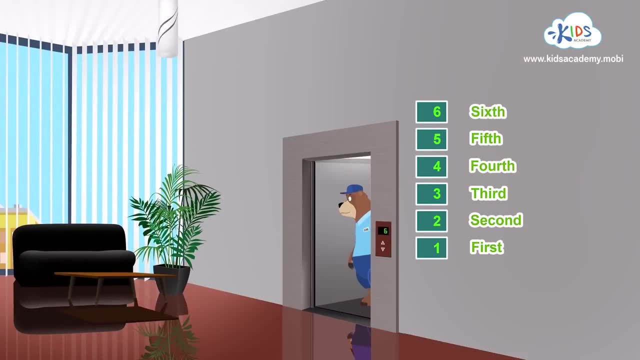 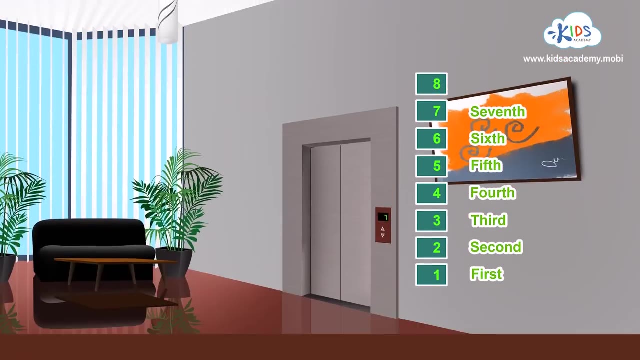 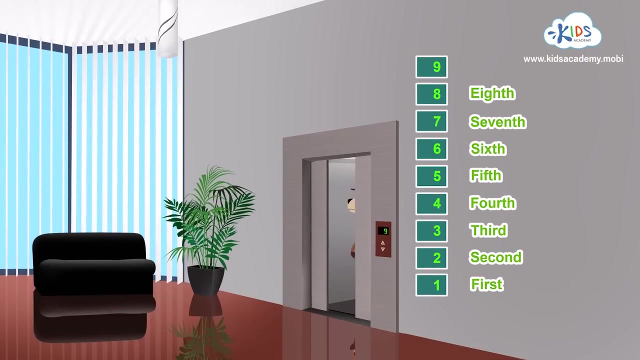 Right, it's the fourth Five, the fifth Six, the sixth Seven, it's the seventh floor. Eight, the ninth Eight. is this the floor I'm looking for? No, it's the ninth floor. Great counting everybody. 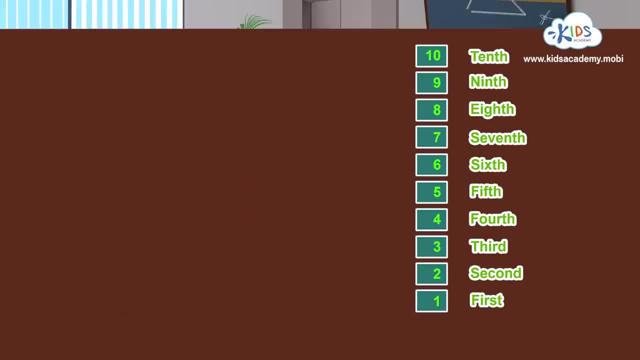 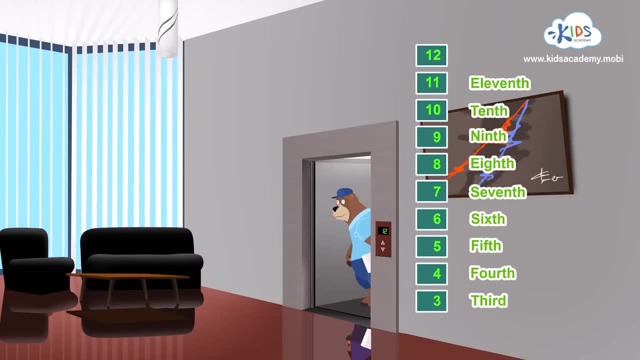 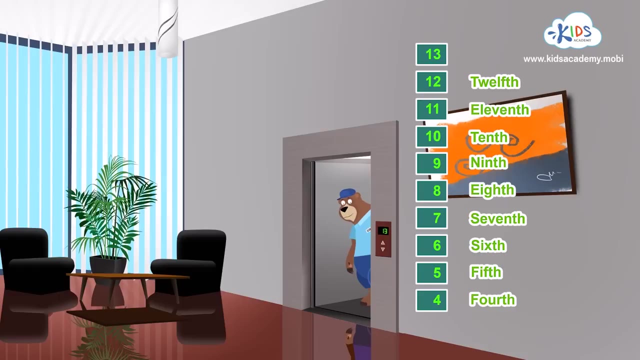 10, the 10th. 11, the 11th. 12, the 12th floor. Which floor are we on now? Right, it's the 13th floor. 14, the 14th floor. 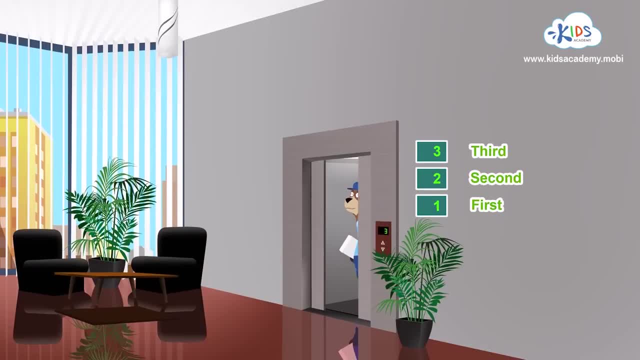 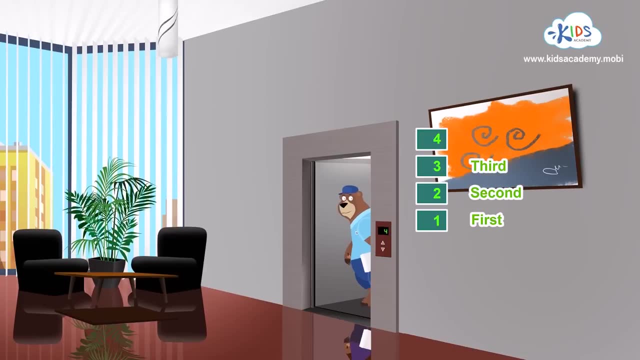 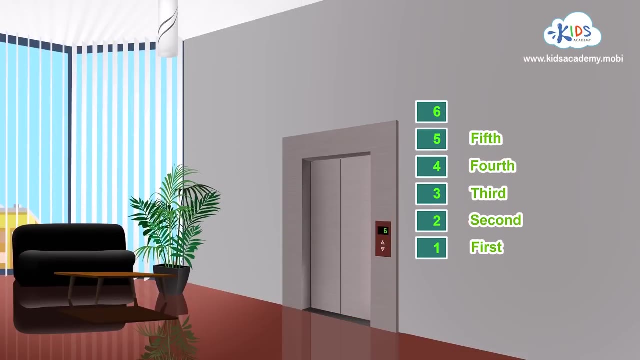 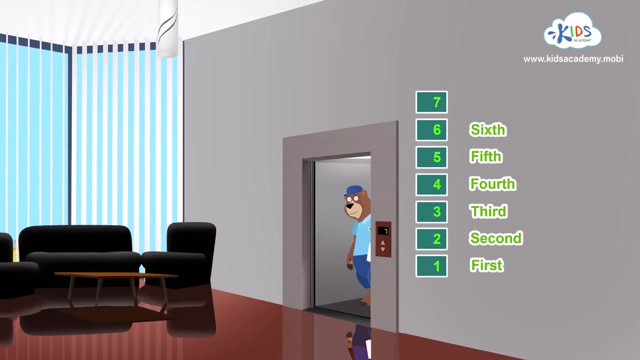 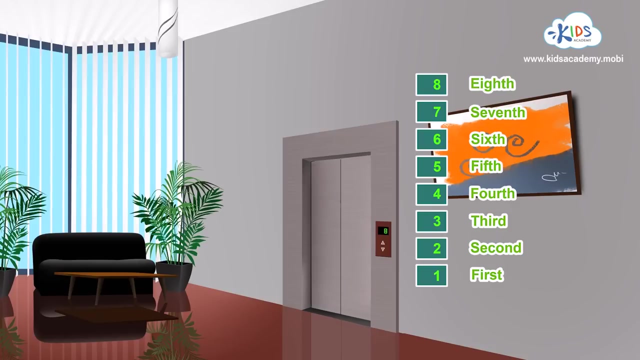 Three: It's the third floor. Four: Which floor is that Right? It's the fourth. Five, The fifth, Six, The sixth, Seven. It's the Eight. The seventh floor, Eight, The eighth. Is this the floor I'm looking for? 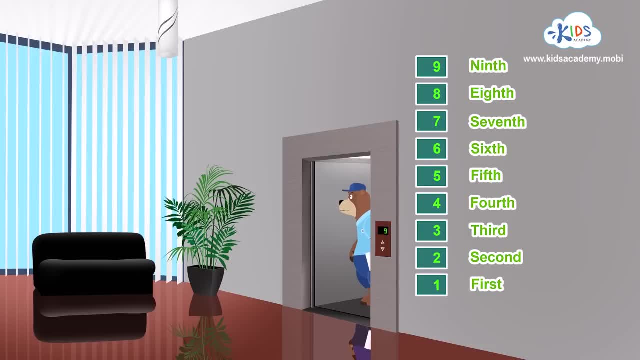 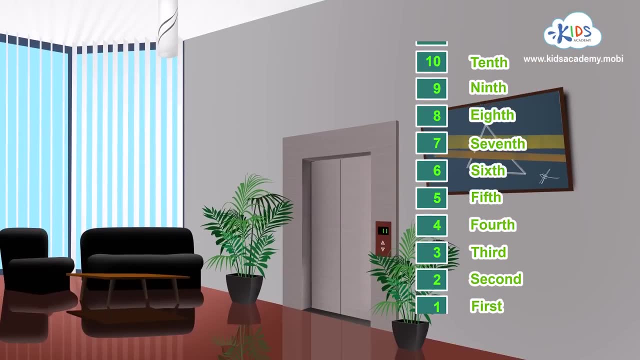 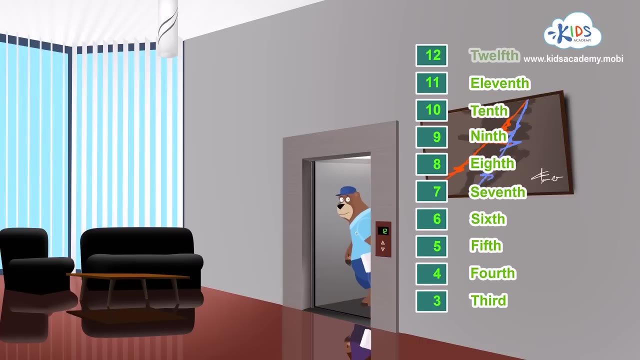 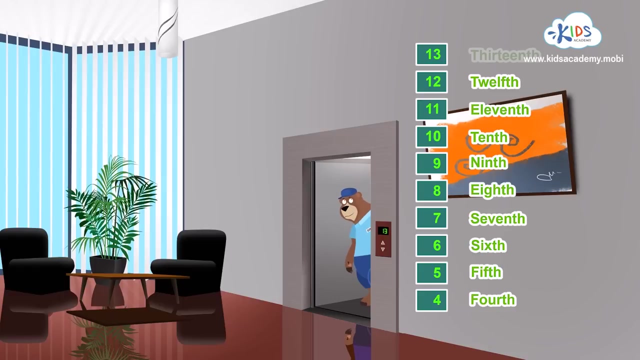 No, It's the ninth floor, Great, counting everybody: Ten, The tenth, Eleven, The eleventh, Twelve, The twelfth floor. Which floor is that? Which floor are we on now? Right, It's the thirteenth floor. 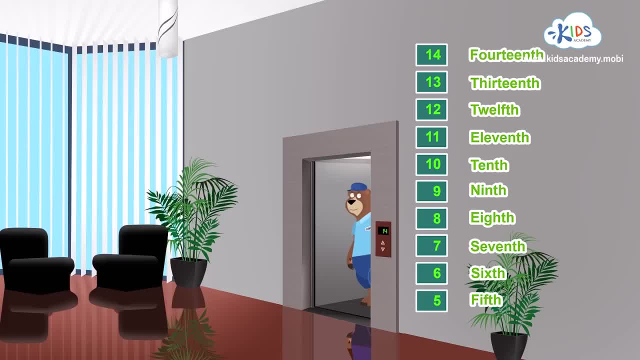 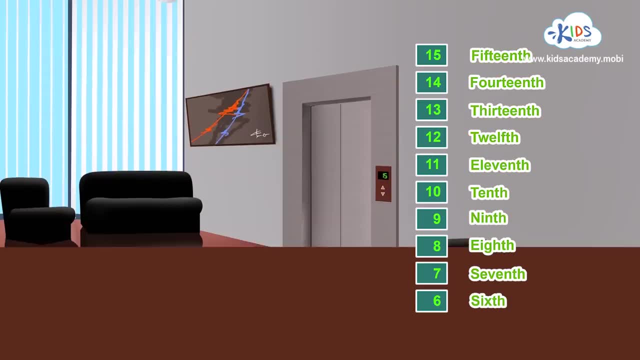 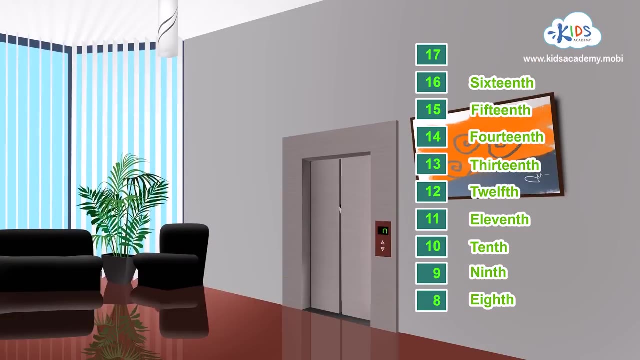 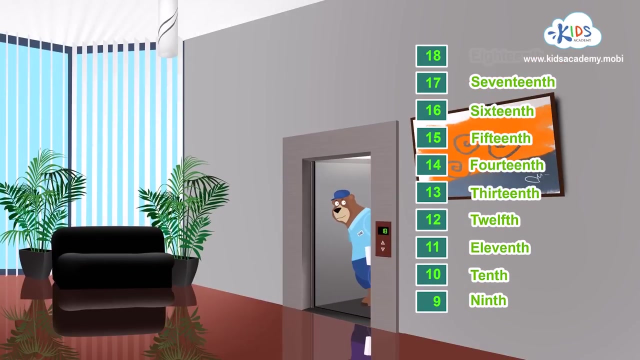 Fourteen, The fourteenth floor. Fifteen, The fifteenth. Sixteen, The sixteenth floor. Maybe this is the twentieth floor. No, It's the seventeenth. Eighteen, The eighteenth floor. Nineteen, The nineteenth. 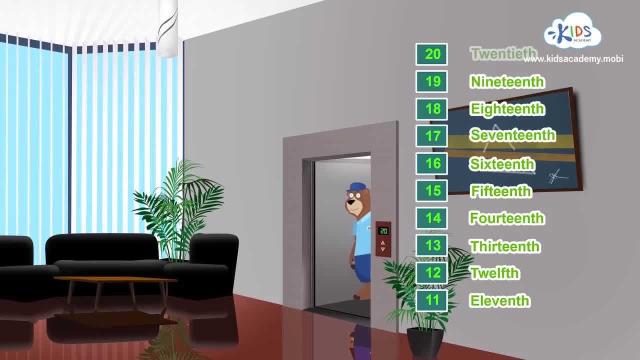 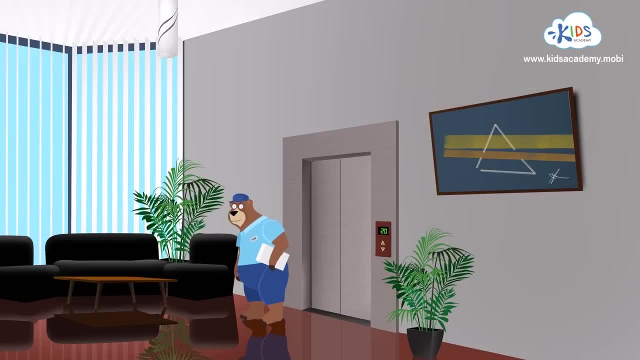 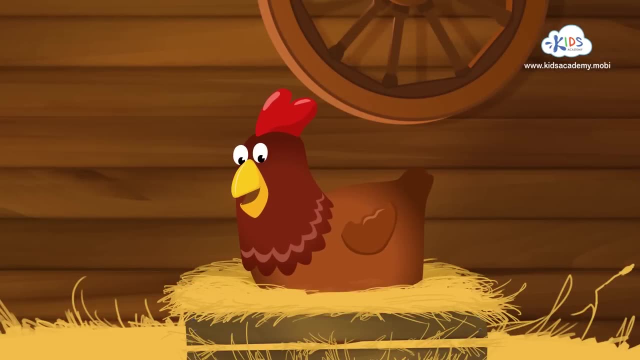 Is this the twentieth floor? All right, We did it. We are on the twentieth floor and I can deliver the parcel. Thanks for helping me count the floors. Bye-bye, Hi there, I'm Chloe, And these are my shiny chicken eggs. 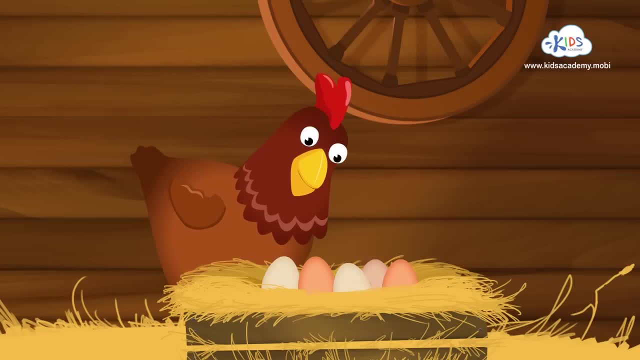 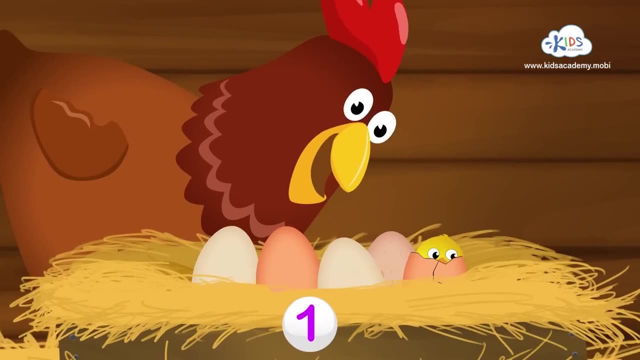 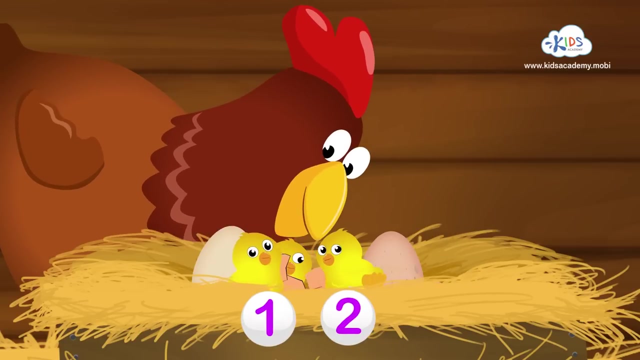 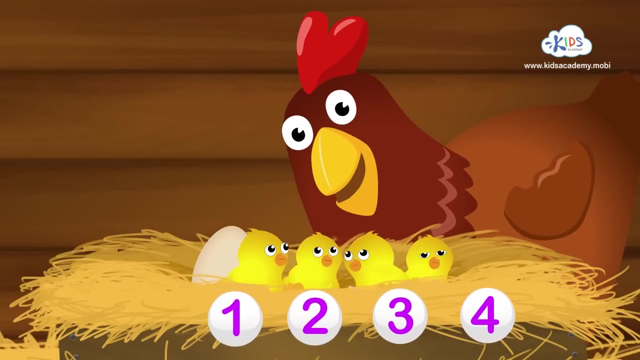 Will you help me count the little chicks as the eggies hatch? You will. Great One, Here's one chick. Two, Now we have two. Three, There are three little chicks now. Four, Now we have four, Five. That's five chicks all together. 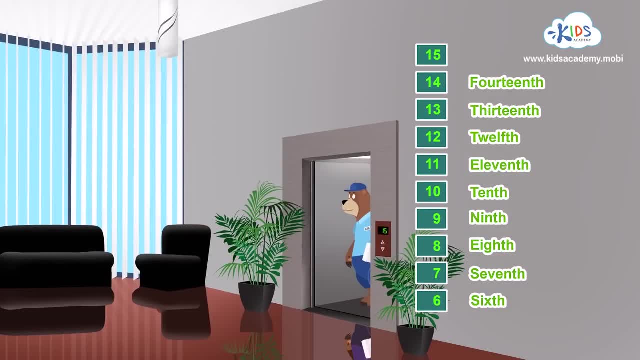 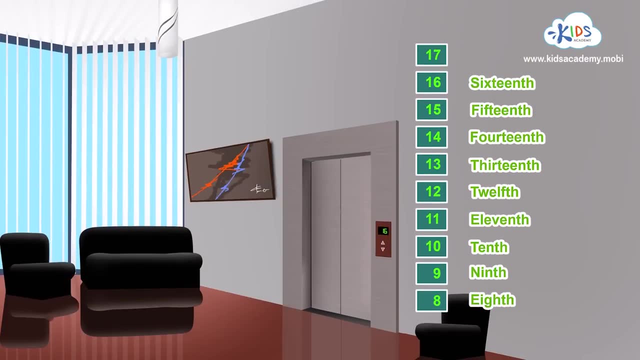 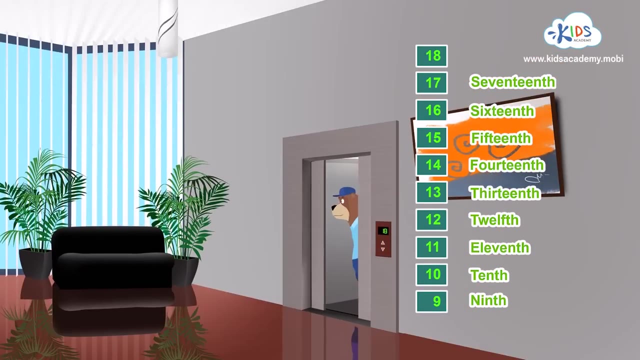 15, the 15th. 16, the 16th floor. Maybe this is the 20th floor. No, it's the 17th. 18, the 18th floor. 19,, the 20th floor. 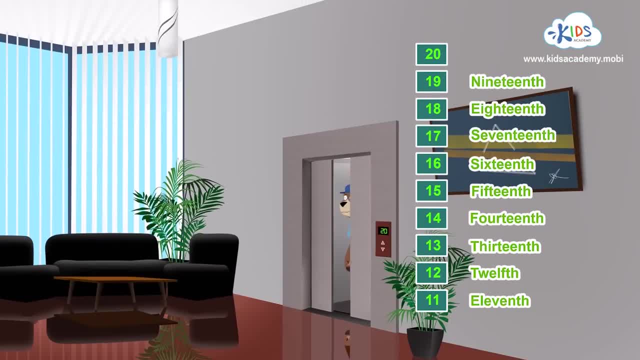 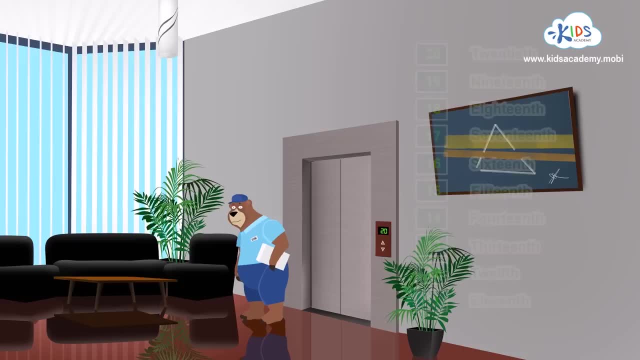 19.. Is this the 20th floor? All right, we did it. We are on the 20th floor And I can deliver the parcel. Thanks for helping me count the floors. Bye-bye. Hi there, I'm Chloe. 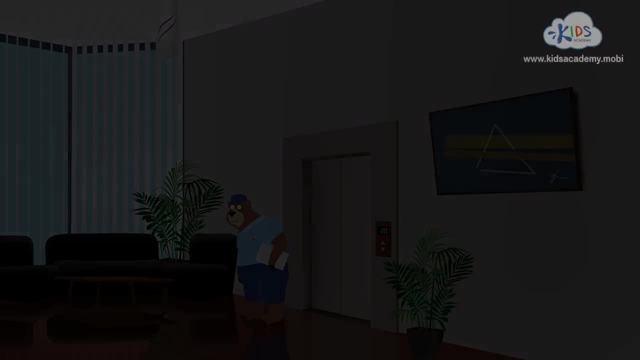 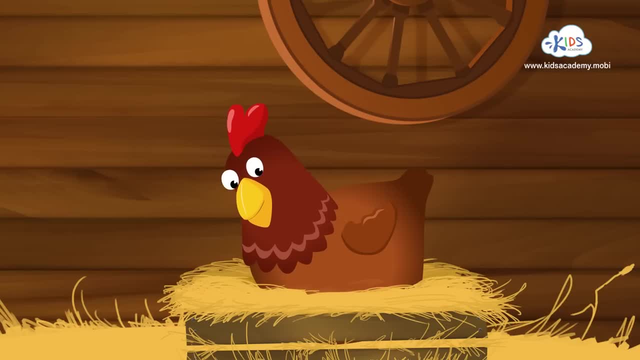 I'm going to count the eggs. I'm going to count the eggs. Oh yeah, I'm going to count the eggs. It's time. I'm going to make the eggs. Oh my, I'm going to make the eggs. 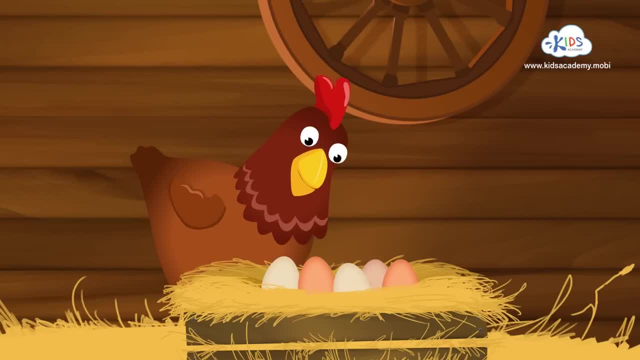 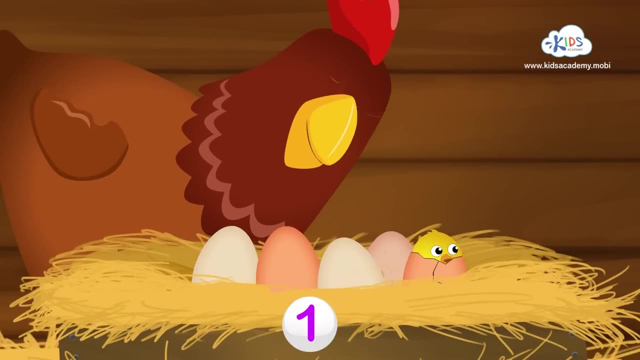 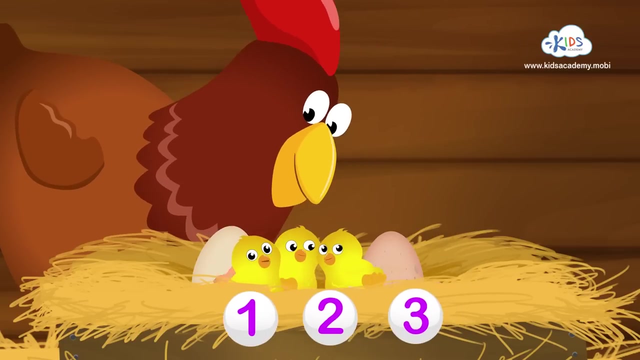 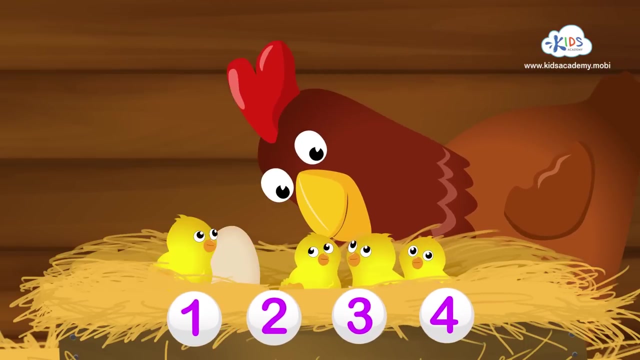 I'm going to make the eggs little chicks as the eggies hatch, You will Great. One, Here's one chick. Two, Now we have two. Three, There are three little chicks, now Four, Now we have four. Five, That's. 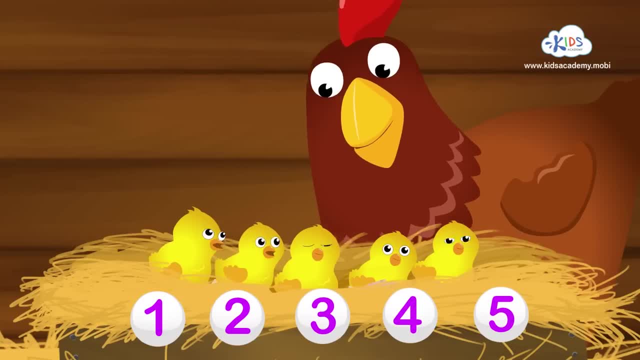 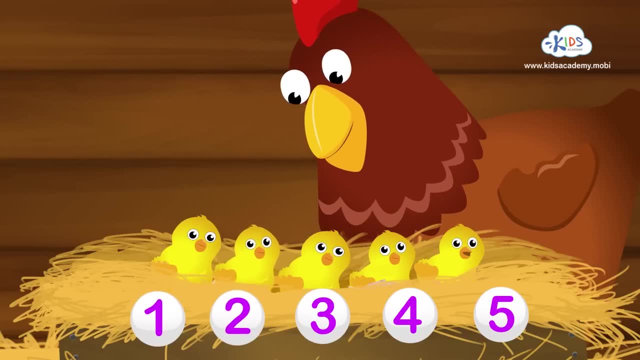 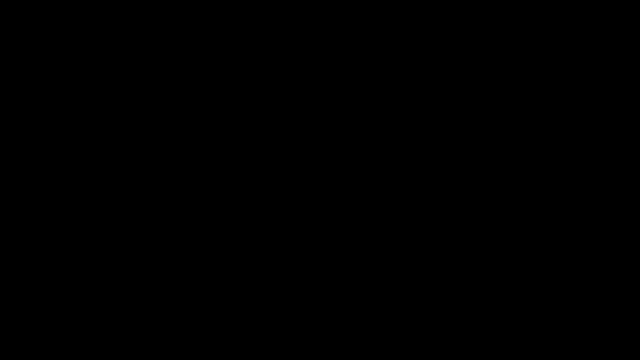 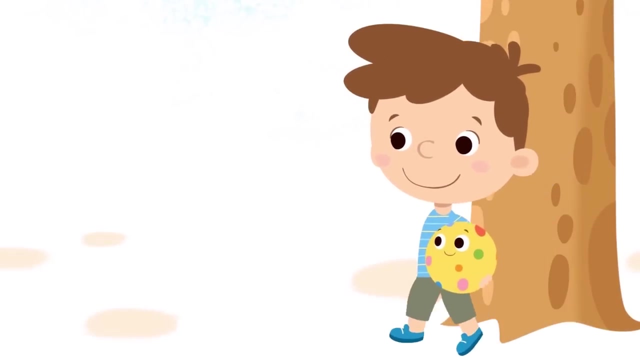 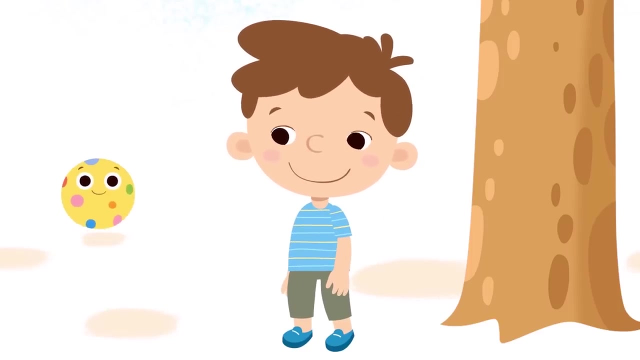 five chicks all together, I've got five cute little chicks. Let's count them again: One, Two, Three, Four, Five. Thanks for helping me count my little chicks, Bye-bye. Hi guys, I'm Michael and this is my friend, Bollie. Bollie and I love to take a walk During. 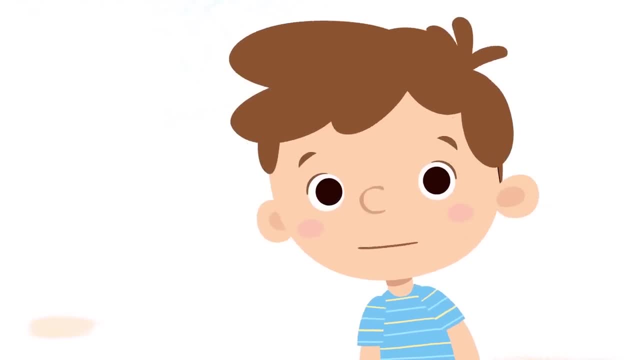 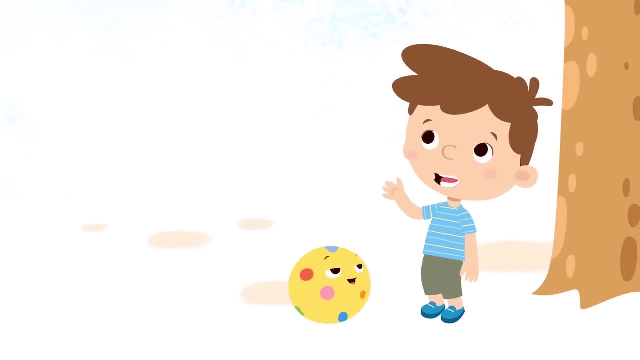 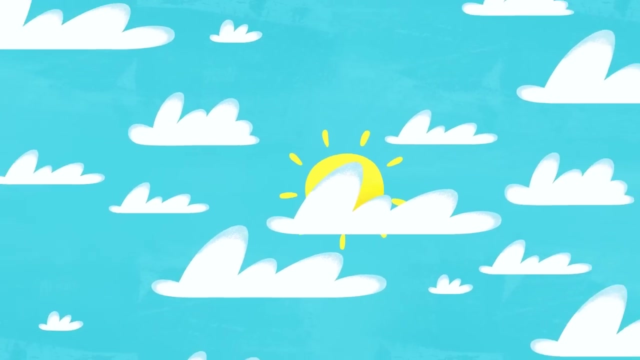 our walks, a lot of interesting things happen. Maybe today something fun will come up too. We need good weather for a walk. There are lots of clouds today. They cover the sun often. How many is lots, I don't know. The sky is so huge It's hard to count. 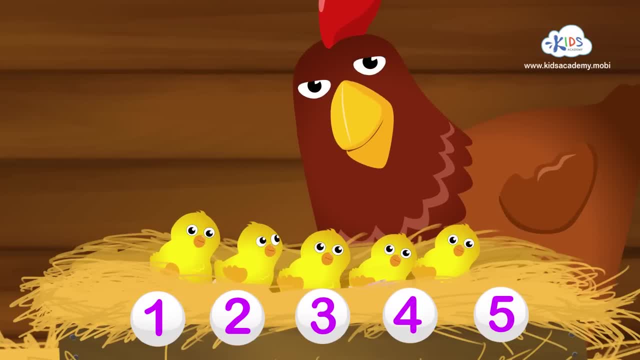 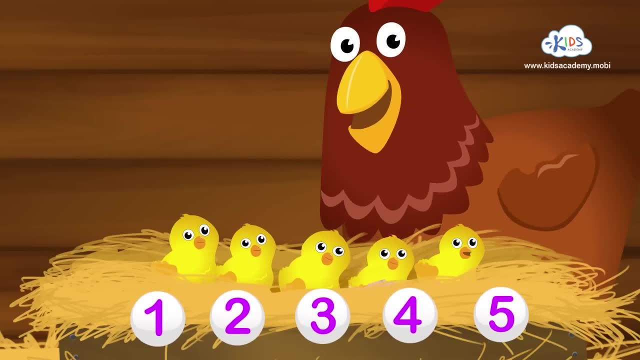 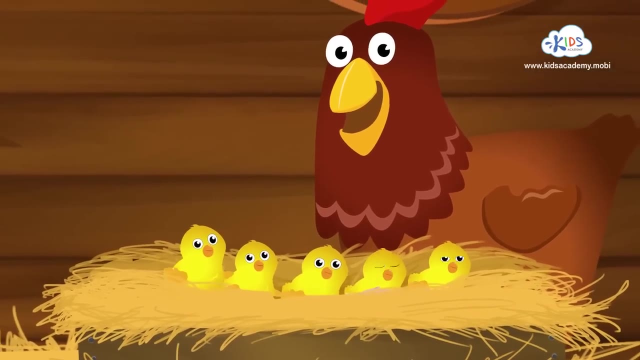 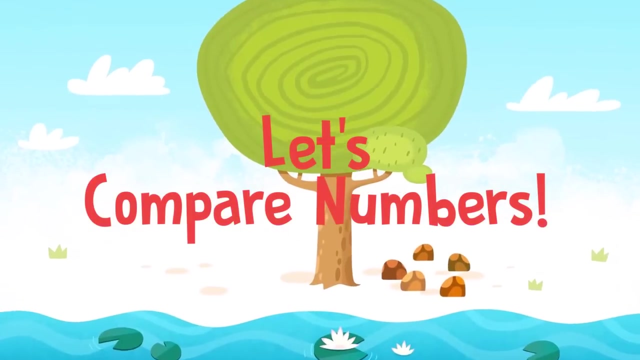 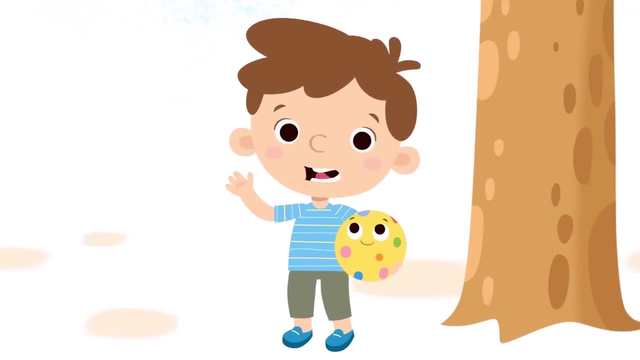 I've got five cute little chicks. Let's count them again: One, Two, Three, Four, Five. Thanks for helping me count my little chicks. Bye-bye, Hi guys. I'm Michael And this is my friend Bally. 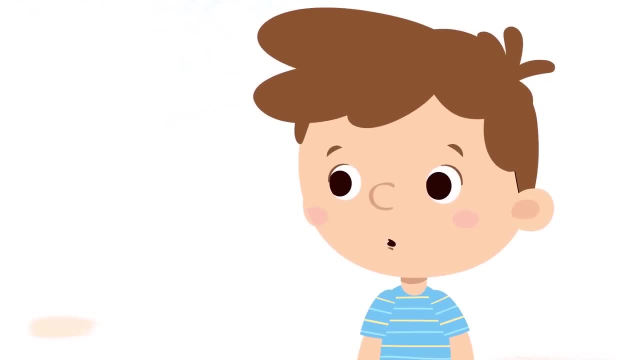 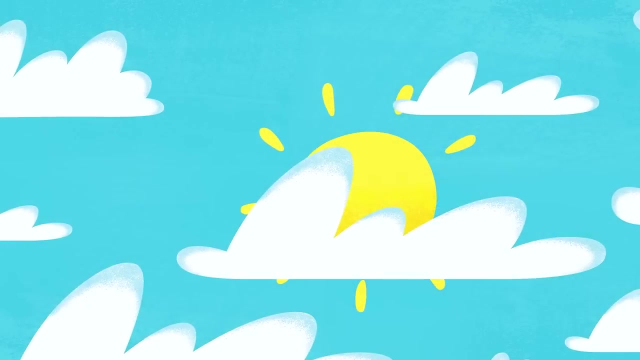 Bally and I love to take a walk. During our walks a lot of interesting things happen. Maybe today something fun will come up too. We need good weather for a walk. There are lots of clouds today. They cover the sun often. 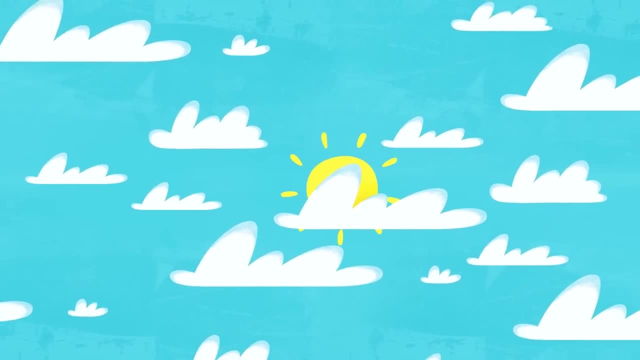 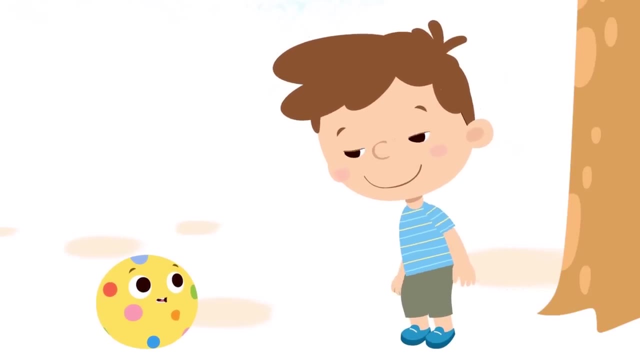 How many is lots? I don't know. The sky is so huge It's hard to count. And how many colorful dots do I have? It's hard to count. them too. You jump very quickly. Well then, let's count these stones. 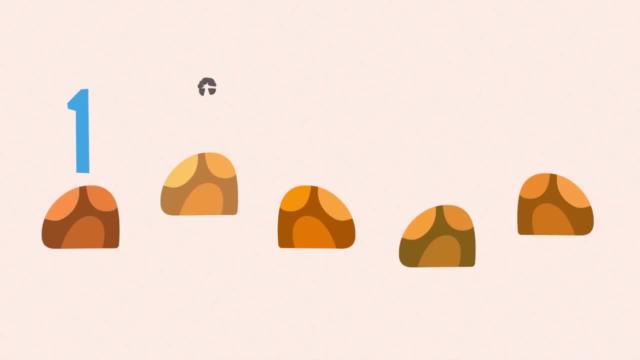 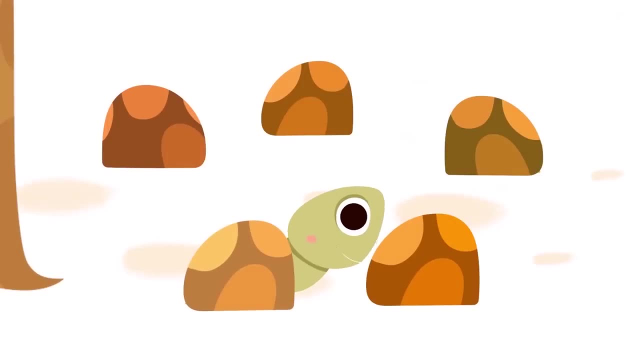 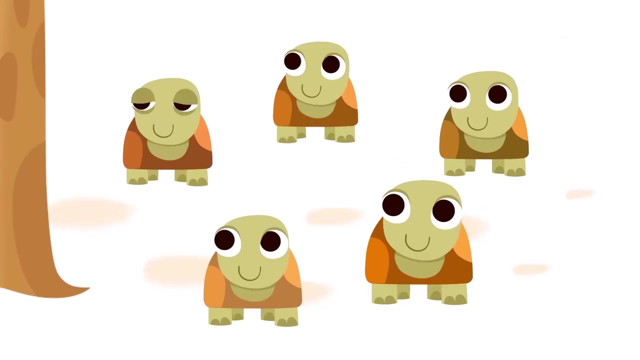 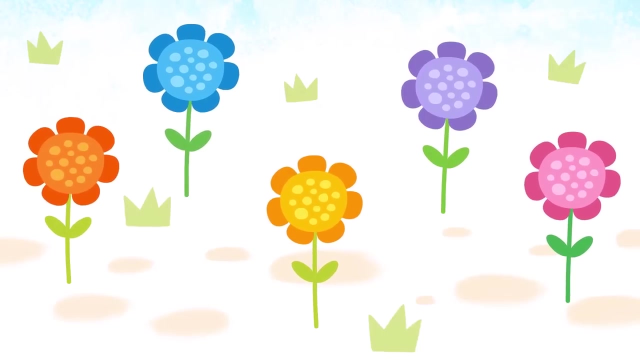 They lie still. One, Two, Three, Four, Five. Wow, They are alive. It's turtles. They are hungry. Let's pick a flower for each of them. Turtles love to eat flowers. Hey, tell us, How many flowers do we need? to treat the turtles? 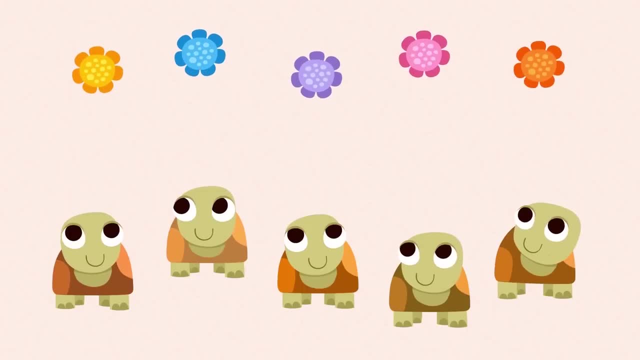 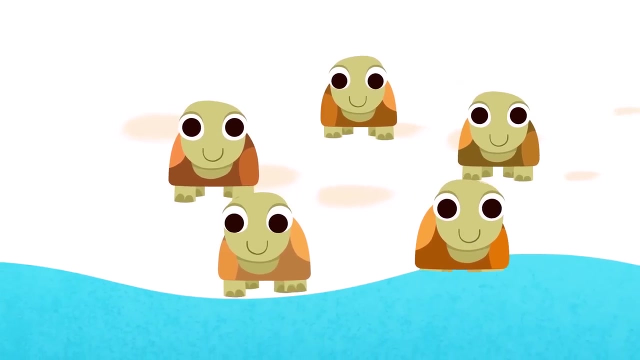 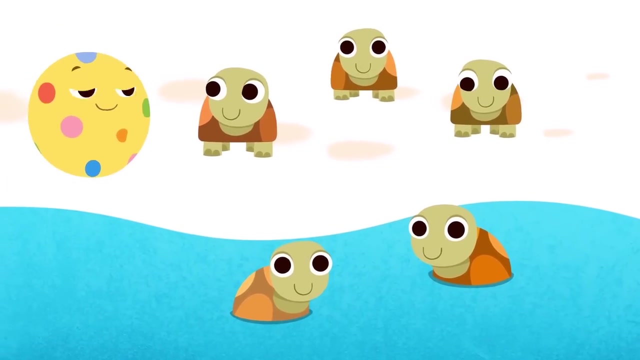 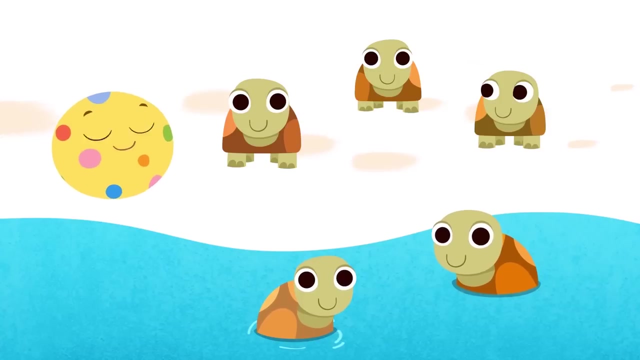 Five, Because there are five turtles: One, Two, Three, Four, Five. Polly solve a problem: How many turtles stay on the shore and how many swim in the water? One, Two, Three. One, Two, Three turtles lie in the grass. 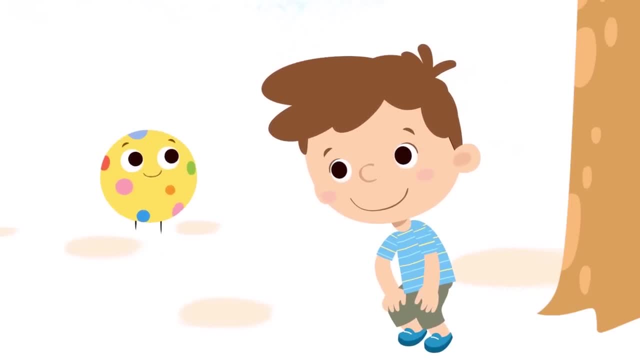 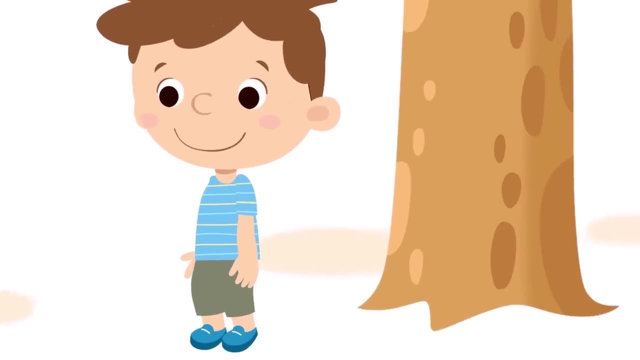 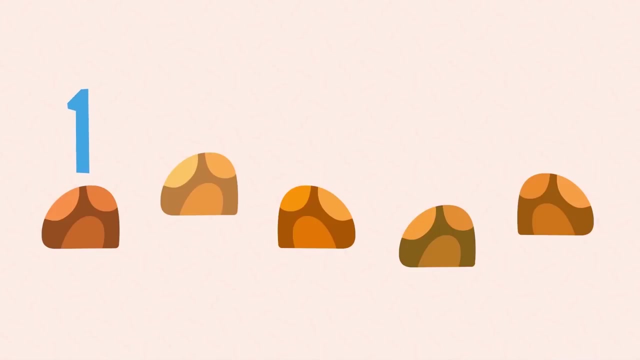 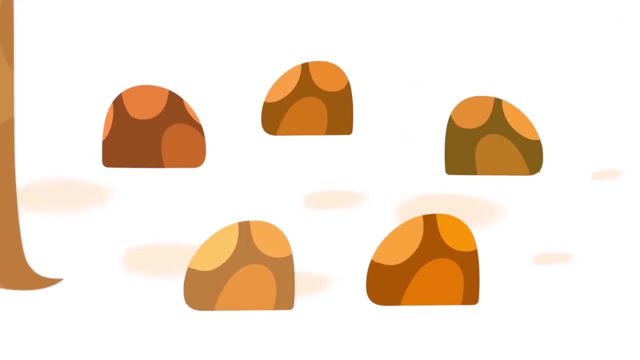 And how many colorful dots do I have? It's hard to count them too. You jump very quickly. Well then, let's count these stones. They lie still. One, Two, Three, Four, Five. Wow, They are alive. 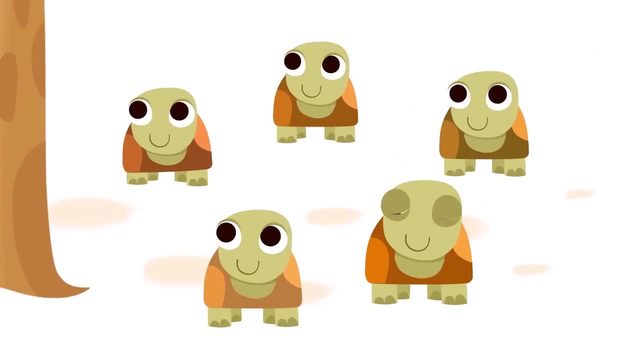 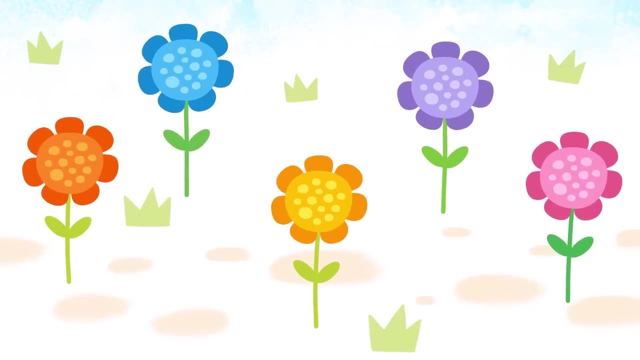 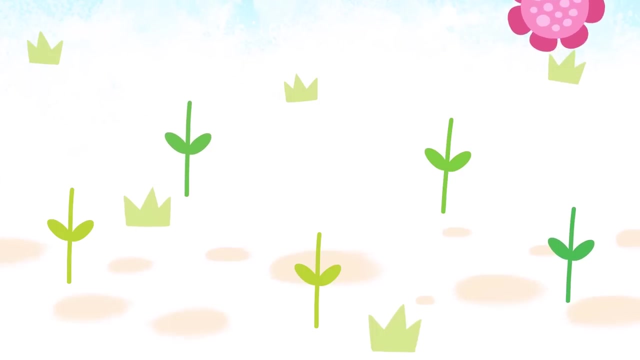 It's turtles. They are hungry. Let's pick a flower for each of them. Turtles love to eat flowers. Hey, tell us, How many flowers do we need to treat the turtles? Five, Because there are five turtles One. 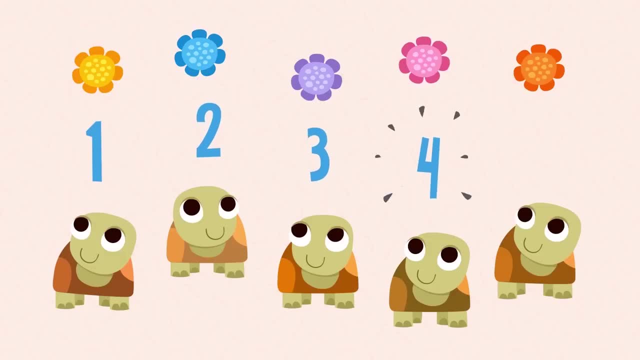 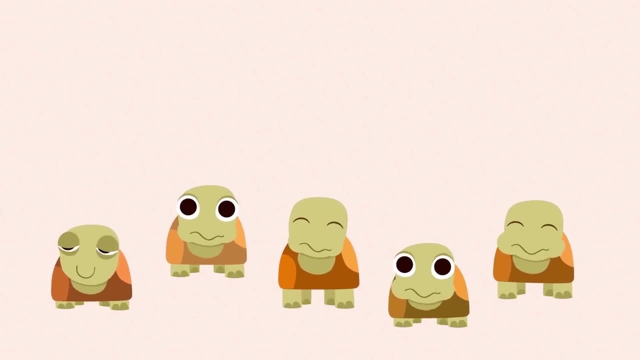 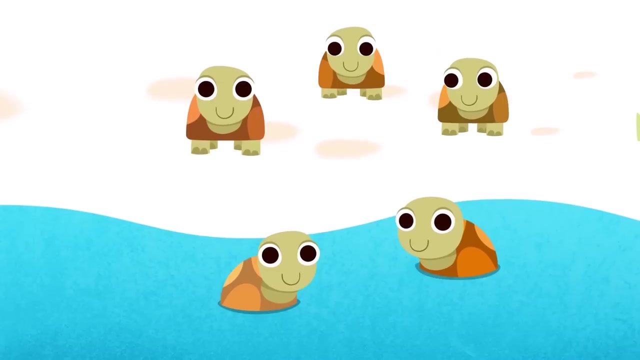 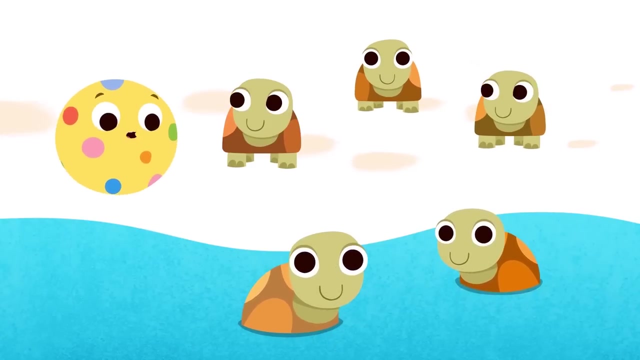 Two, Three, Four, five. Polly solve a problem: How many turtles stay on the shore and how many swim in the water? One, two, three, One two, Three turtles lie in the grass and two turtles are in the water. 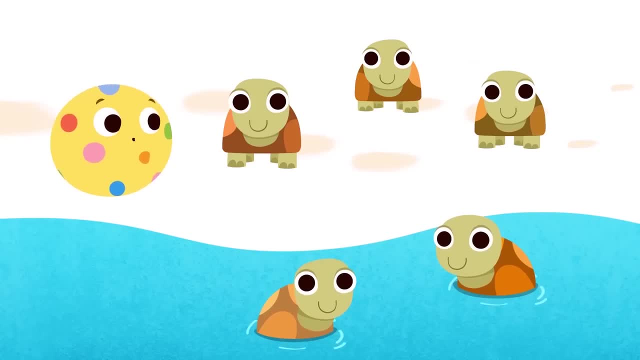 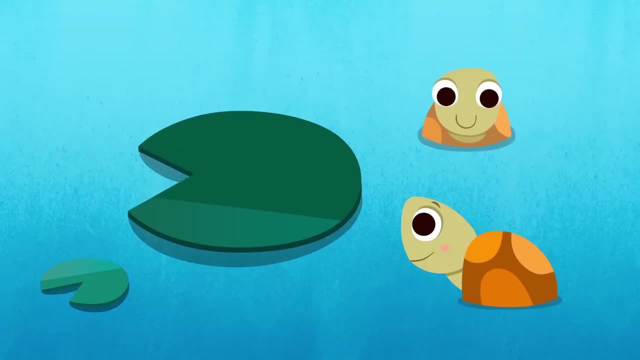 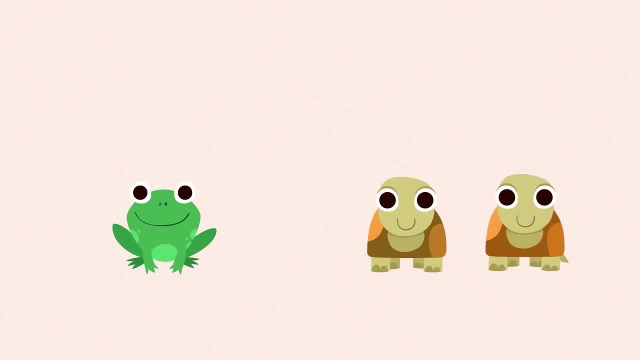 Which number is larger? There are more turtles in the grass, so I think number three is larger than number two. Number two is not the smallest. Number one is smaller. There's one frog and there are two turtles. They have more fun than the lonely frog. 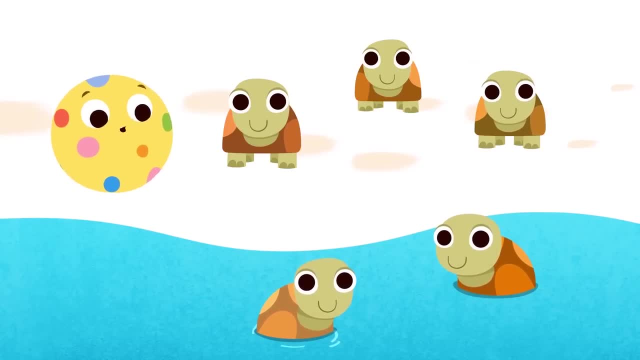 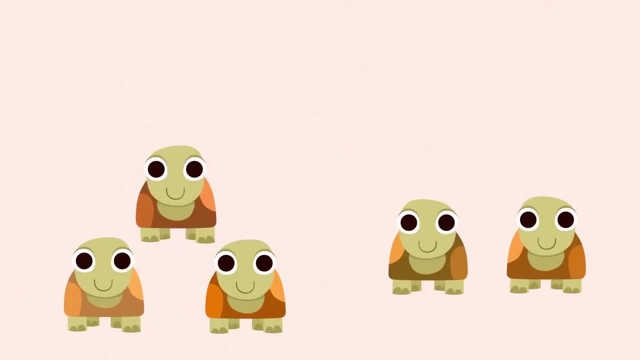 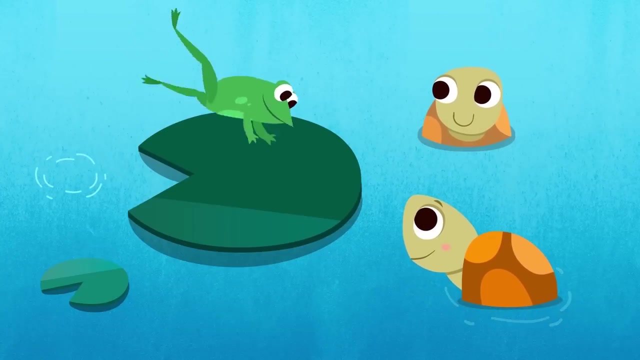 And two turtles are in the water. Which number is larger? There are more turtles in the grass, So I think number three is larger than number two. Number two is not the smallest. Number one is smaller. There's one frog and there are two turtles. 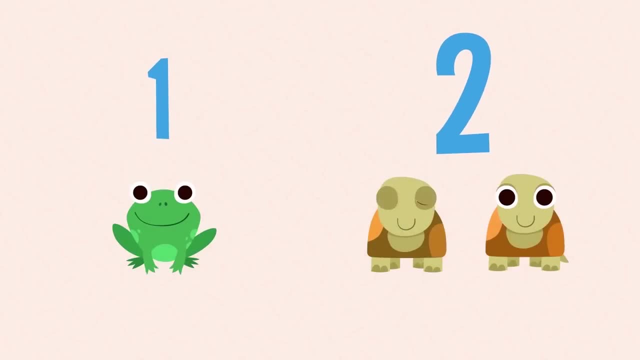 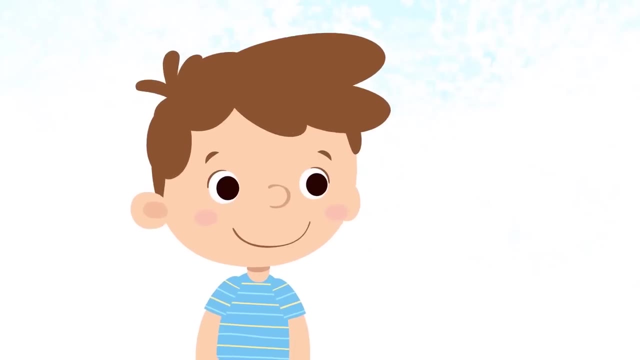 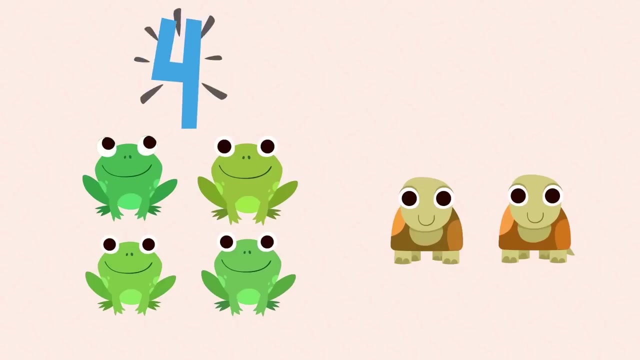 They have more fun than the lonely frog. The frog wasn't bored for long. Now there's a whole crowd of frogs here. Right Now there are more frogs than turtles in the stream, Because there are four frogs and only two turtles. number four is larger than number two. 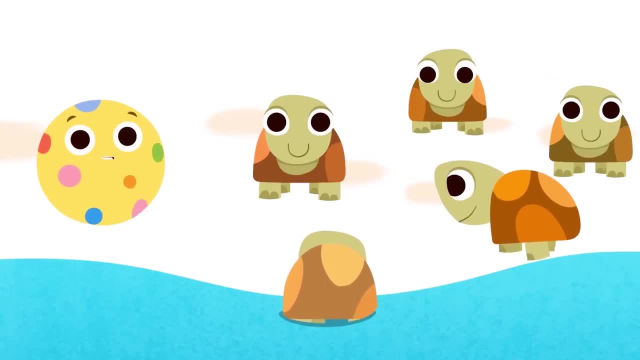 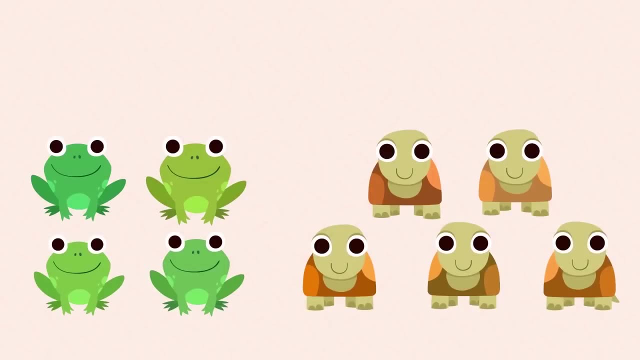 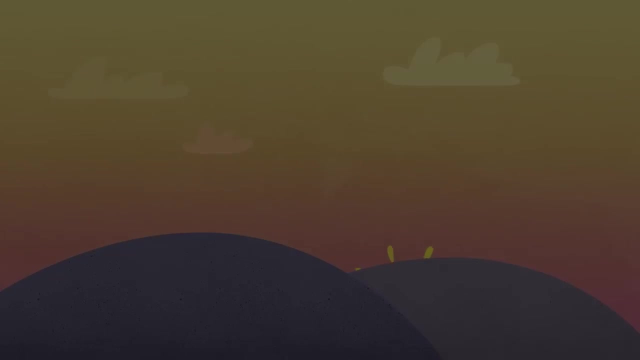 And what if we compare all the turtles and all the frogs? Who will be more? There are more turtles. There are five of them, And there are just four frogs. Number five is larger. It's evening, It's time to go home. 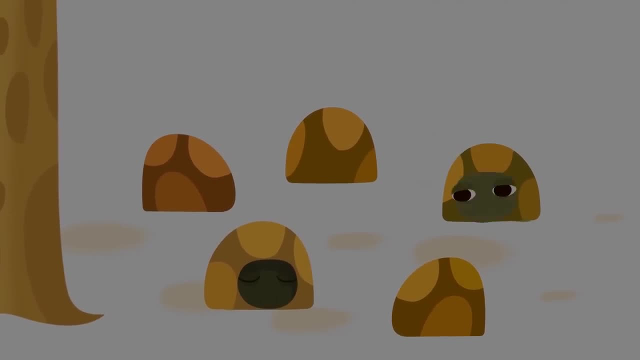 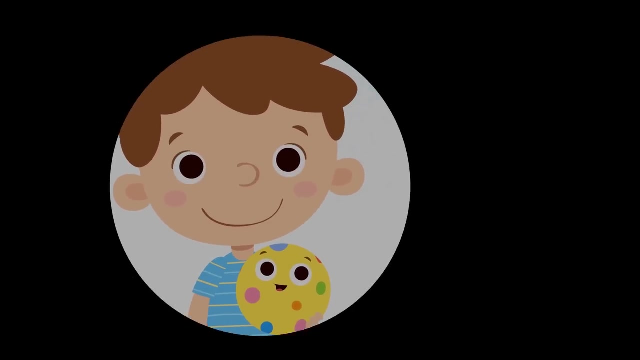 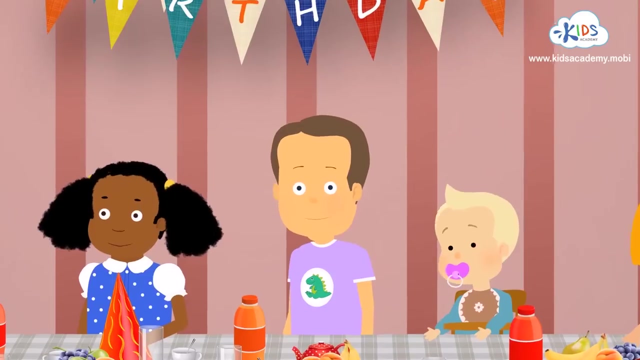 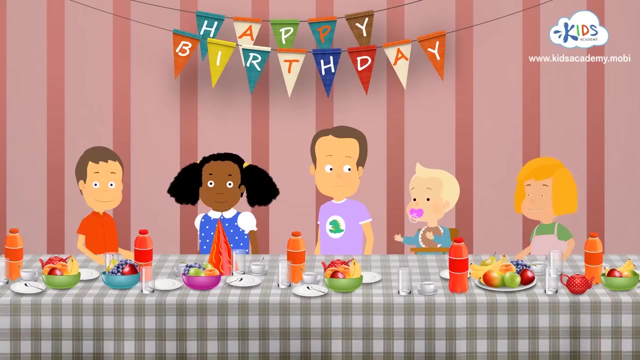 Tomorrow will bring a new day and new interesting stories. Bye guys, See you soon. Hey everybody, I'm Matt And these are my friends Charlotte, Andy, Zoe and little Benny. We have our birthday today. What better way to celebrate a birthday than with a sweet cake and a few candles? 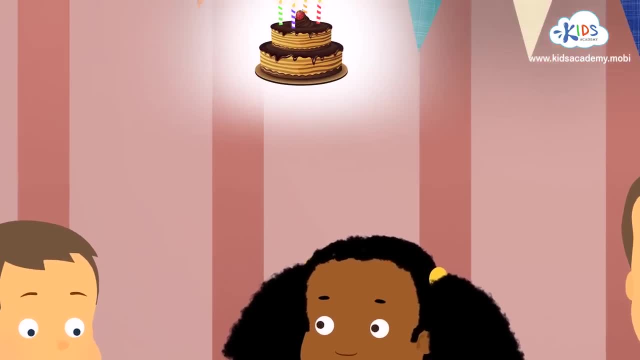 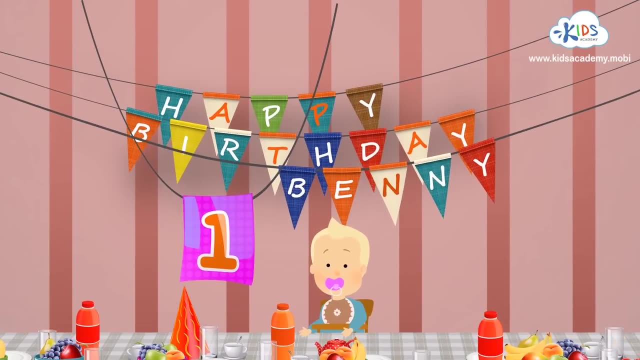 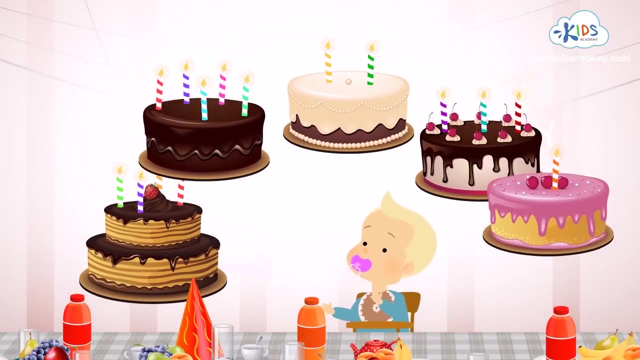 Oh my, Somebody's mixed up our cakes. Can you find the right cake for each of us? I'm one year old today, So my cake has one candle on it. Can you see any cakes with one candle Right? This is my birthday cake. 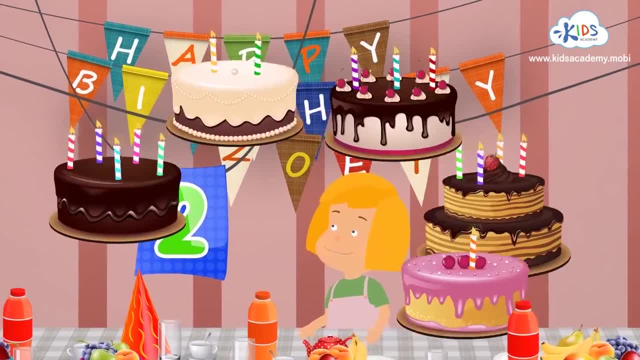 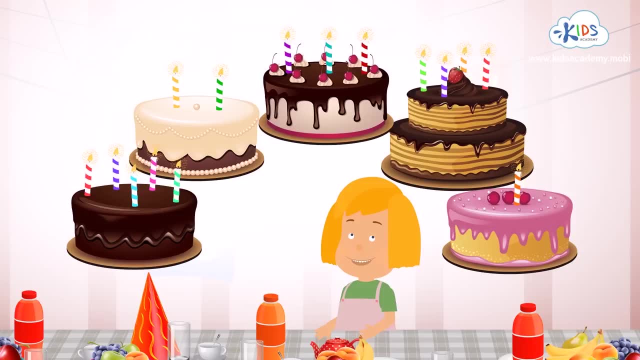 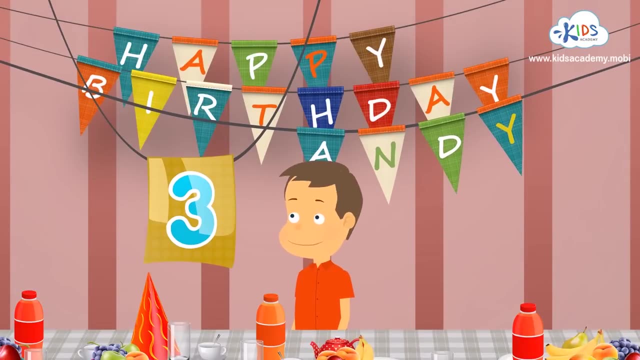 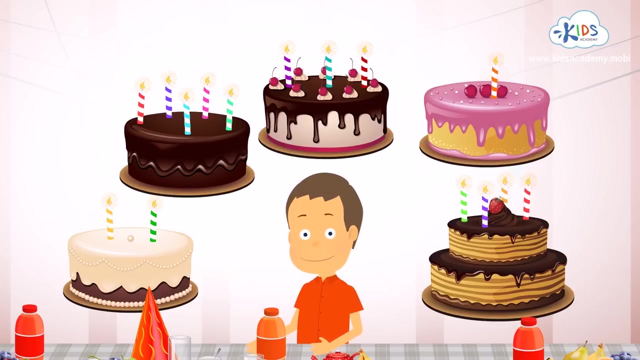 I'm two today, So my birthday cake has how many candles? Two candles. Where is the cake with two candles? Here it is. I'm three today, So there are how many candles on my cake? Three, And my cake is this one. 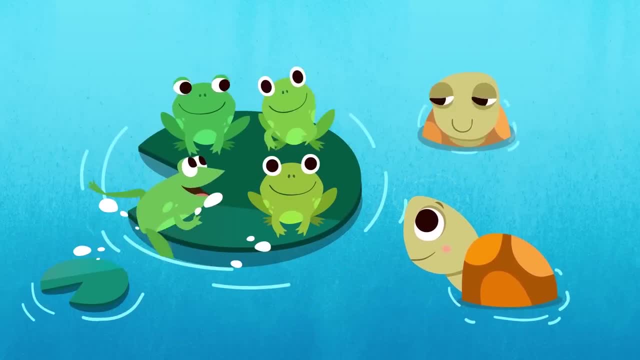 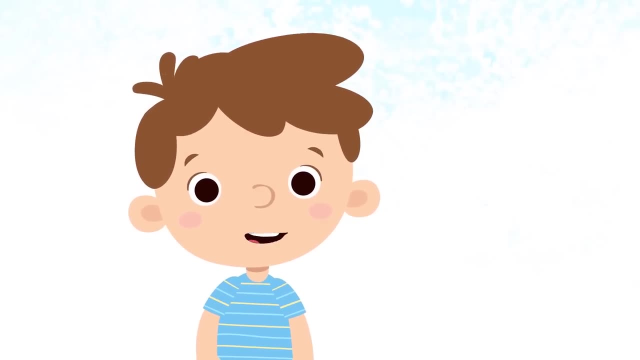 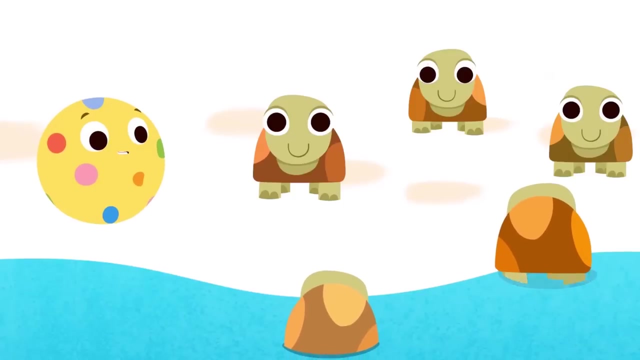 The frog wasn't bored for long. Now there's a whole crowd of frogs here. Right Now there are more frogs than turtles in the stream, Because there are four frogs and only two turtles. number four is larger than number two. And what if we compare all the turtles and all the frogs? 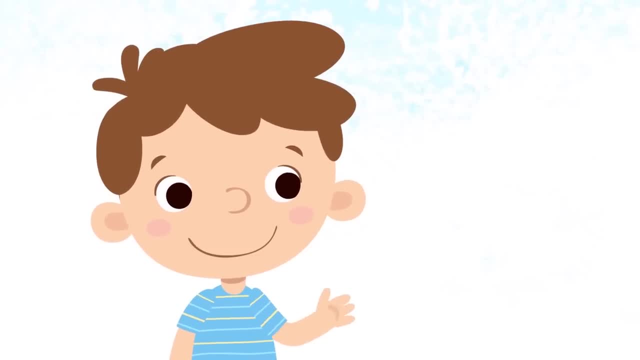 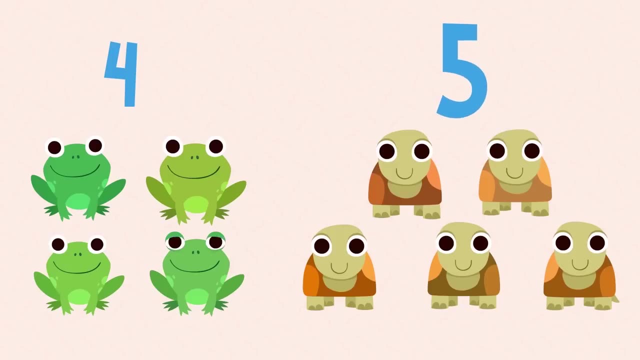 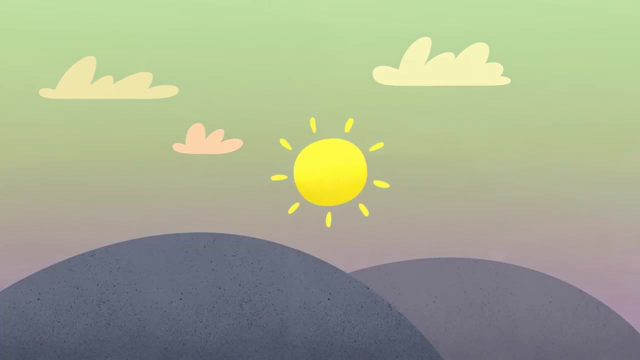 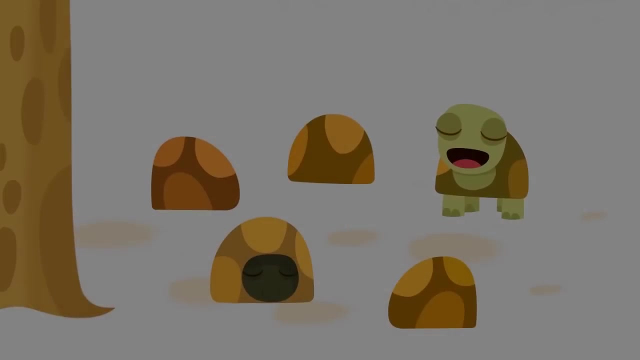 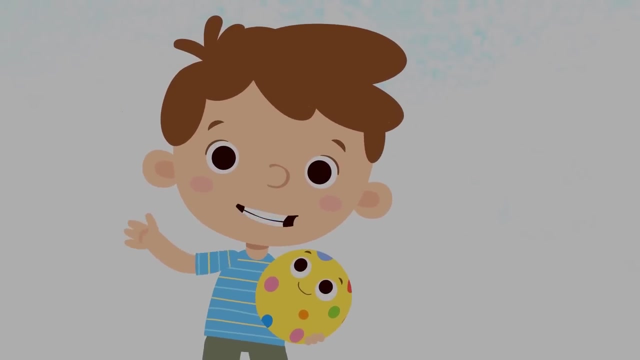 Who will be more? There are more turtles. There are five of them, and there are just four frogs. Number five is larger. It's evening. It's time to go home. Tomorrow will bring a new day and new interesting stories. Bye guys. 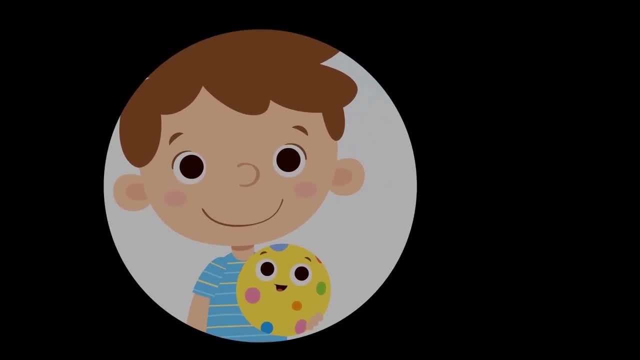 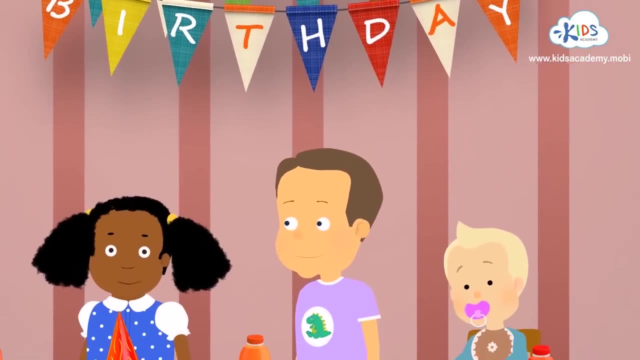 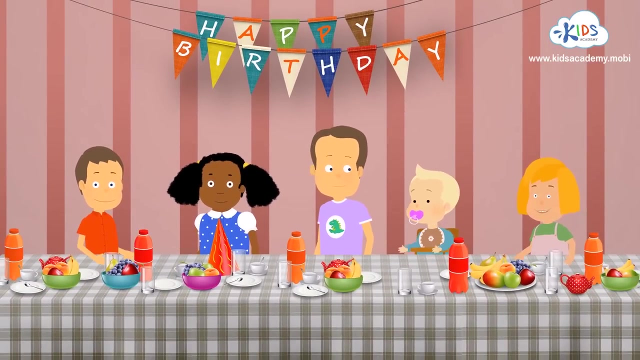 See you soon. Hey everybody, I'm Matt, And these are my friends Charlotte, Andy, Zoe and little Benny. We have our birthday today. What better way to celebrate a birthday than with a sweet cake and a few candles? 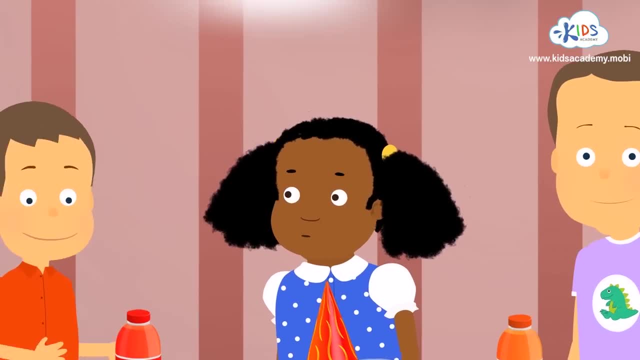 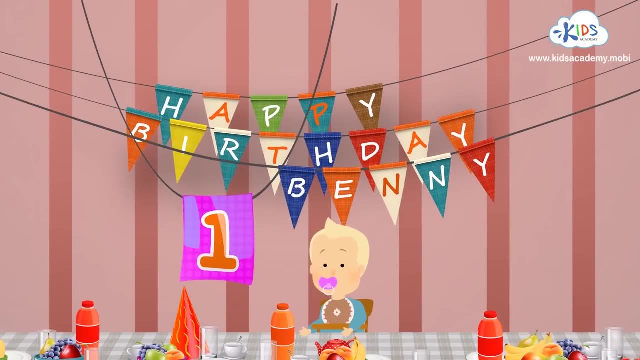 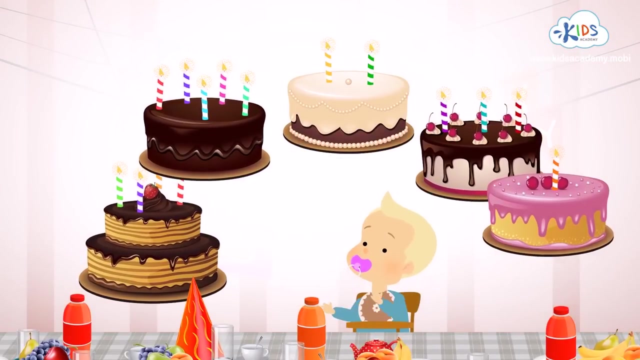 Oh my, Somebody's mixed up our cakes. Can you find the right cake for each of us? I'm one year old today, So my cake has worn out. My cake has one candle on it. Can you see any cakes with one candle? 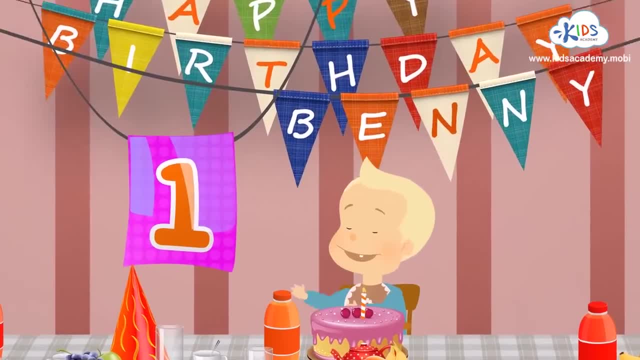 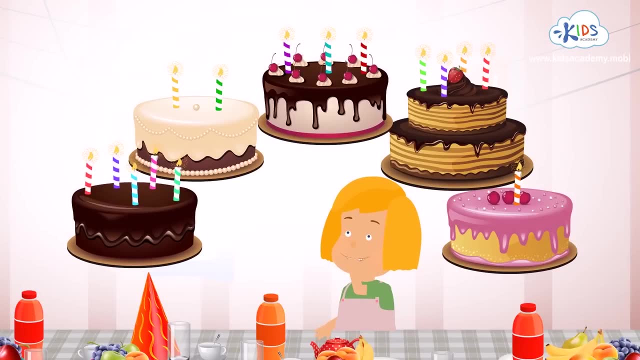 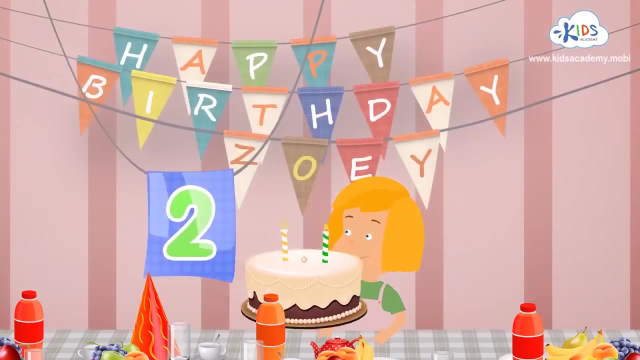 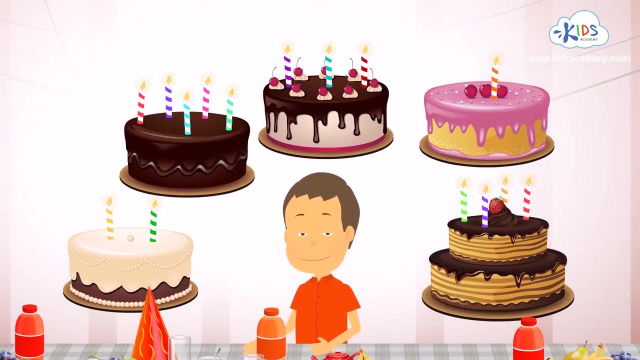 Right, This is my birthday cake. I'm two today, So my birthday cake has how many candles? Two candles. Where is the cake with two candles? Here it is. I'm three today, So there are how many candles on my cake? 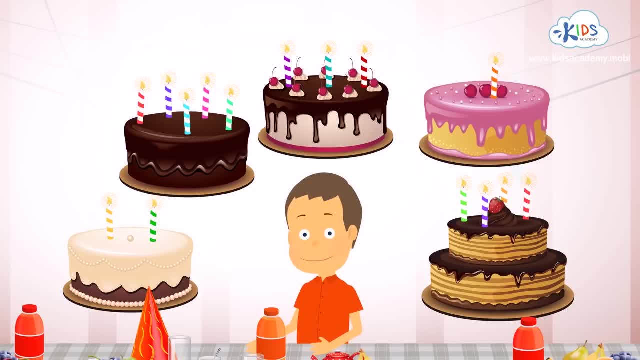 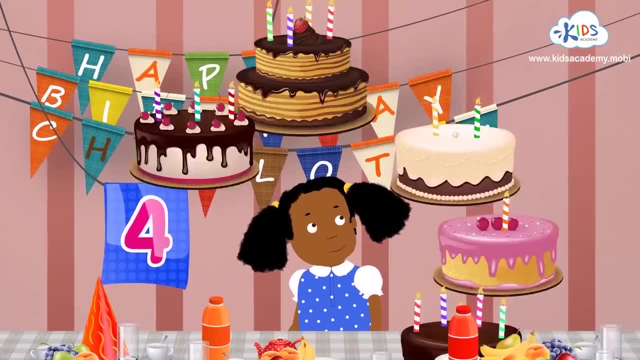 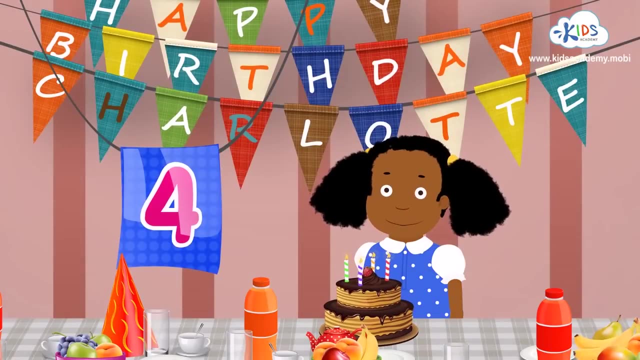 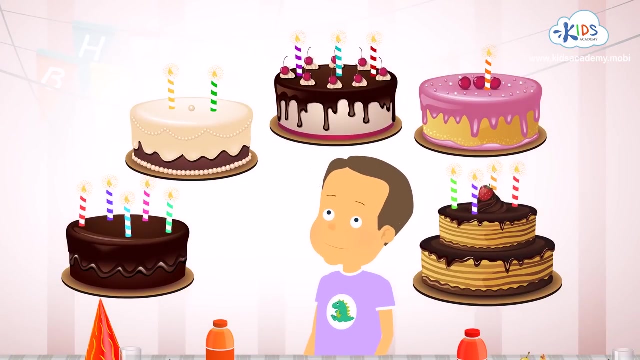 Three, And my cake is this one. I'm four today. Can you see a cake with four sparkling candles on it, Right? This is my cake. I'm five today And a cake with five candles is this one, Hooray. 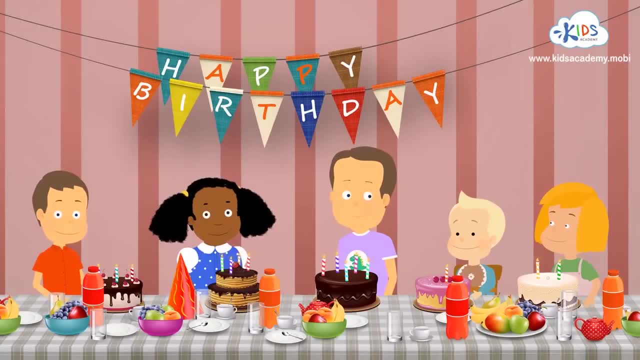 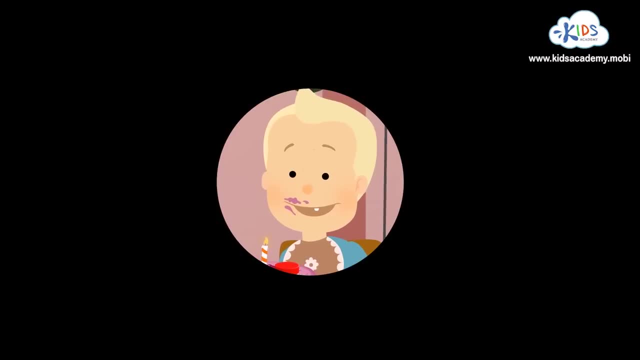 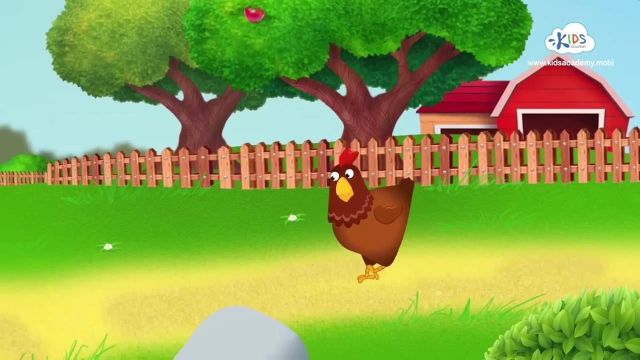 We've got our birthday cakes and we're ready for our birthday party. Everybody shout: happy birthday. Hi, I'm Chloe and I'm in big trouble. I've lost my five little chickens. Will you help me find and count my lost chicks? 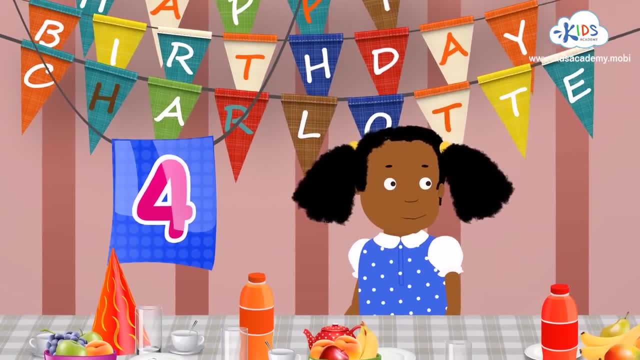 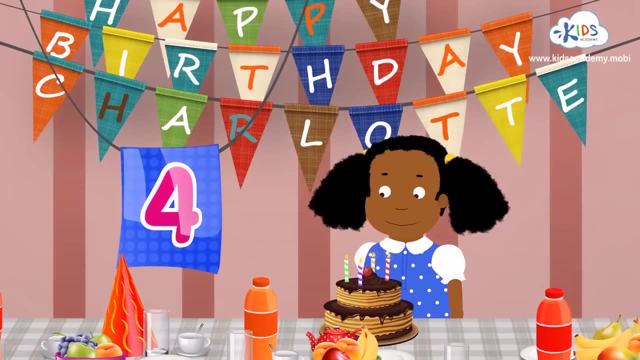 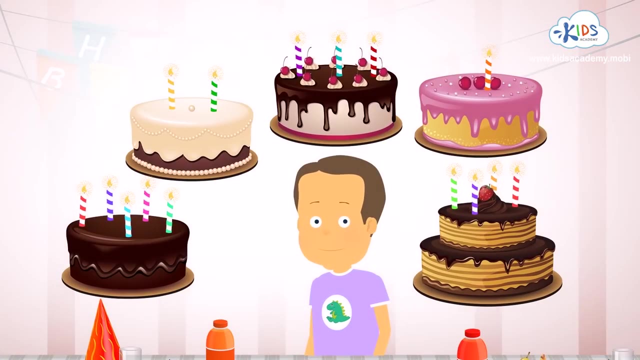 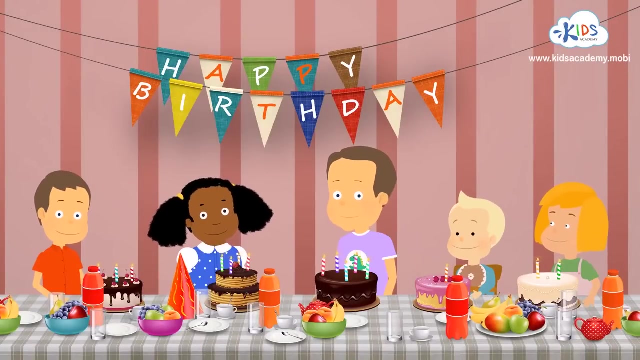 I'm four today. Can you see a cake with four sparkling candles on it? Right, This is my cake. I'm five today And a cake with five candles is This one, This one. Hooray, We've got our birthday cakes and we're ready for our birthday party. 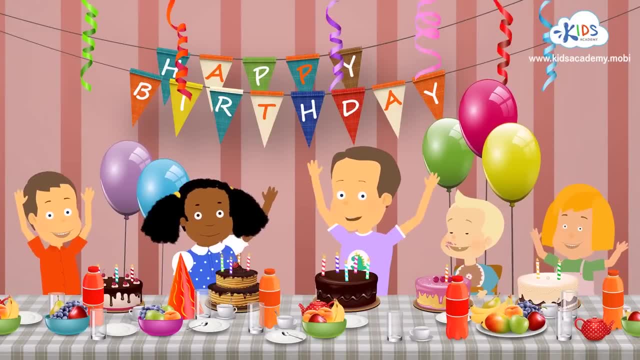 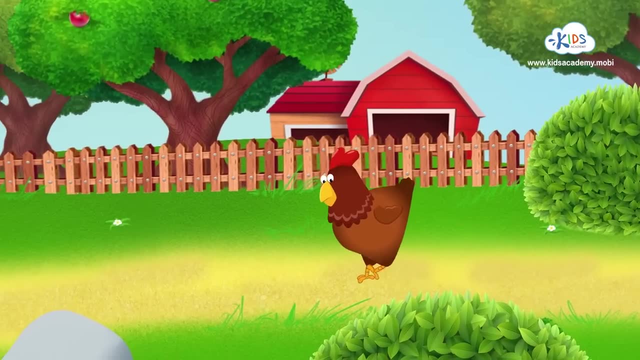 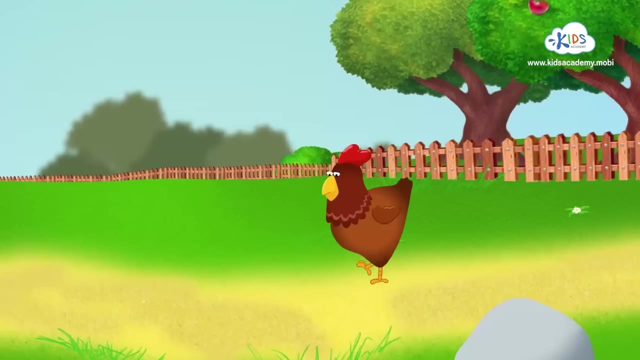 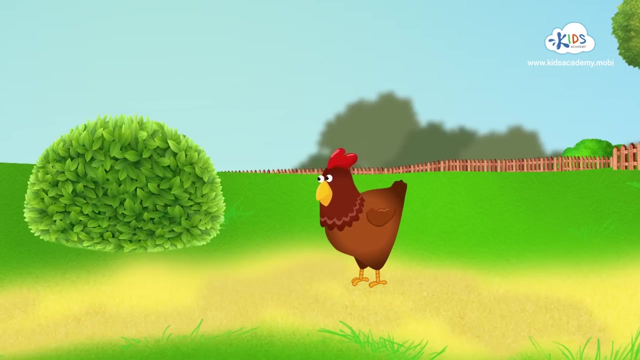 Everybody shout: happy birthday. Hi, I'm Chloe and I'm in big trouble. I've lost my five little chickens. Will you help me find and count my lost chicks? You will Great. Hmm, I wonder where my chicks could be hiding. 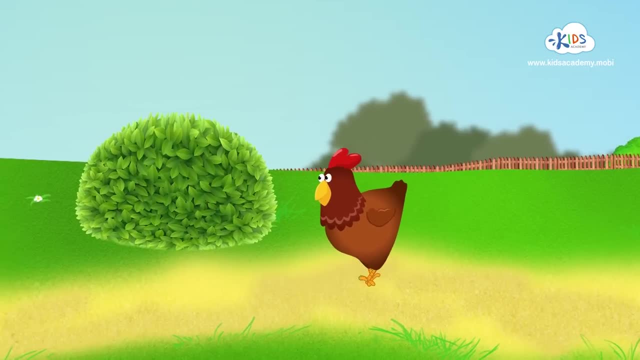 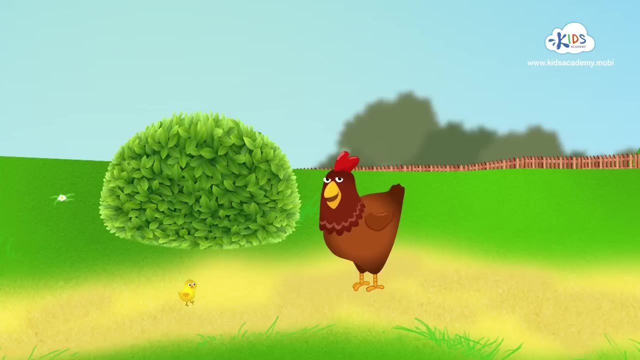 Maybe behind those bushes, Great Count with me. We've found One little chick. See any more chickens? Right, There's one in the grass. That's, That's, That's, That's, That's, That's. 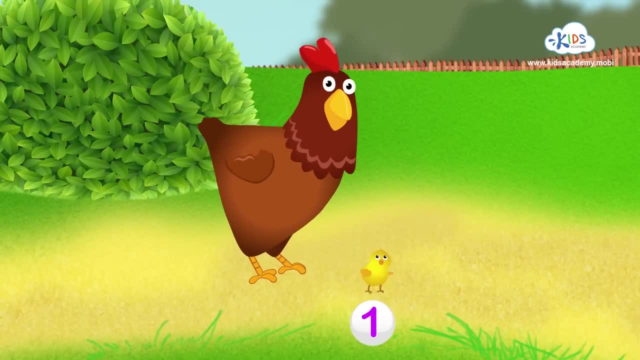 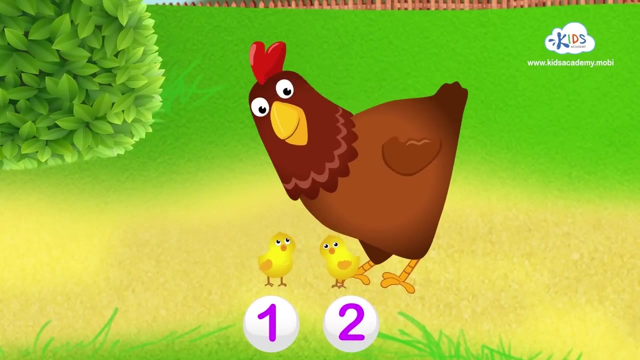 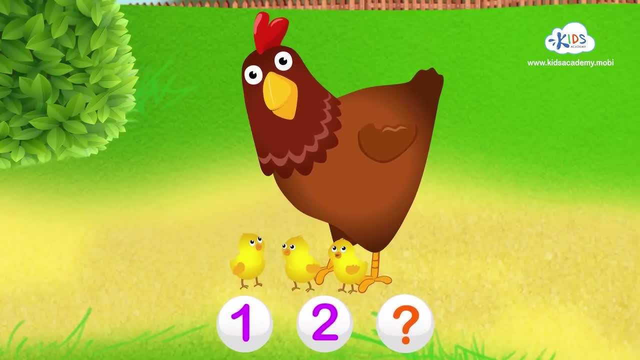 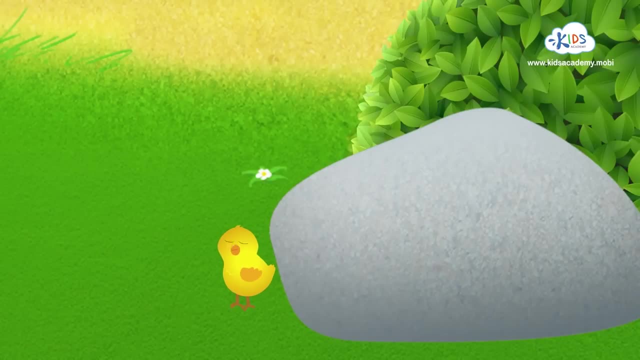 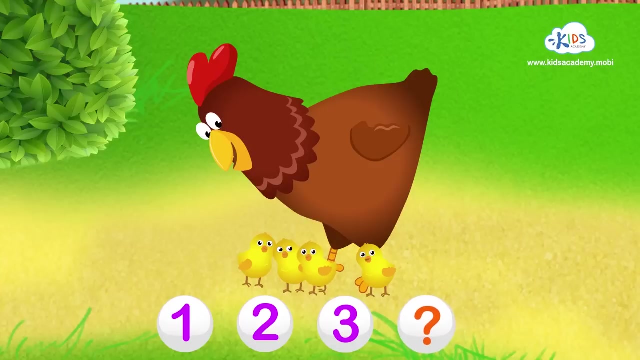 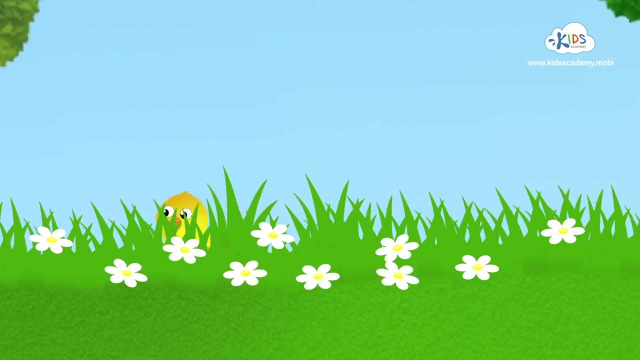 We've got Three little chickens now. Great job, Let's go have a peek behind that big stone. That's, That's. That's, That's Four. And the littlest chick is right in the flower bed. Great, That's. 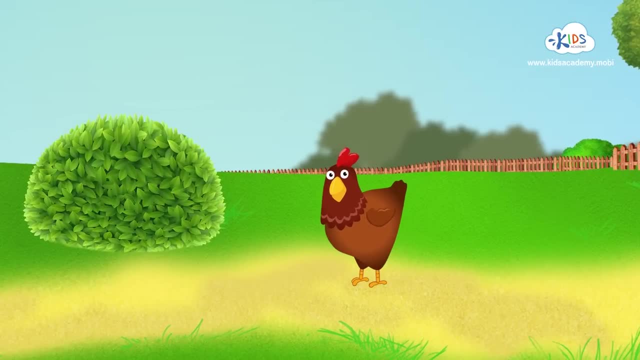 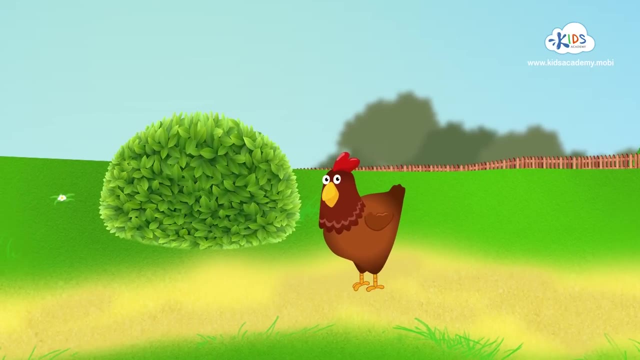 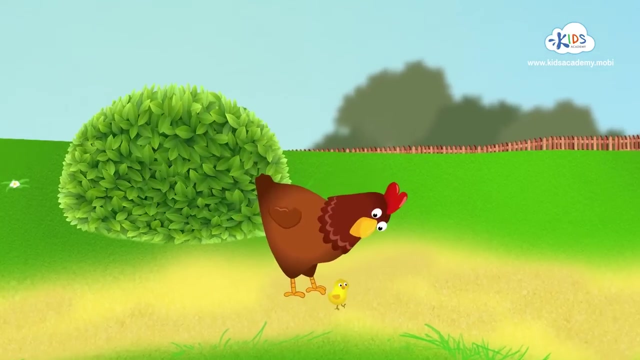 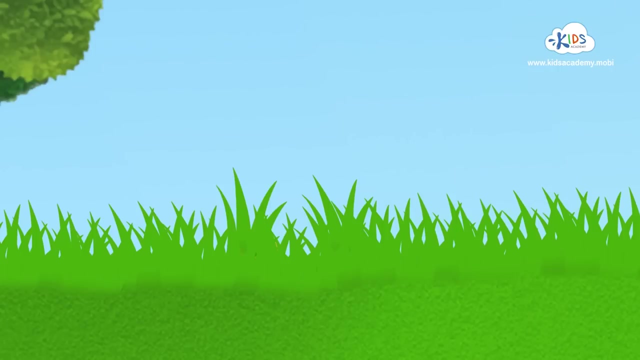 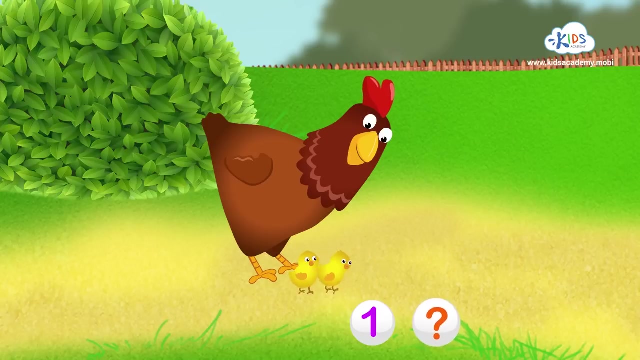 You will Great. Hmm, I wonder where my chicks could be hiding, Maybe behind those bushes? Great Count with me. We've found one little chick. See any more chickens? Right, There's one in the grass, That's. 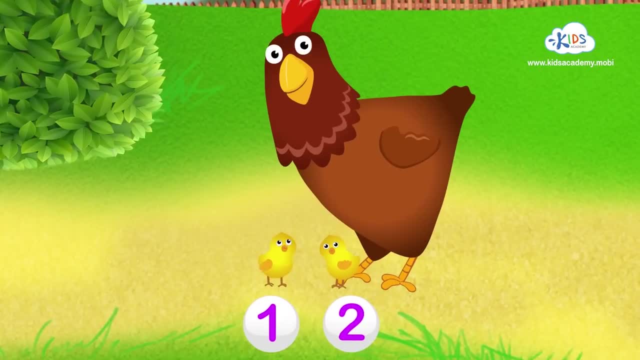 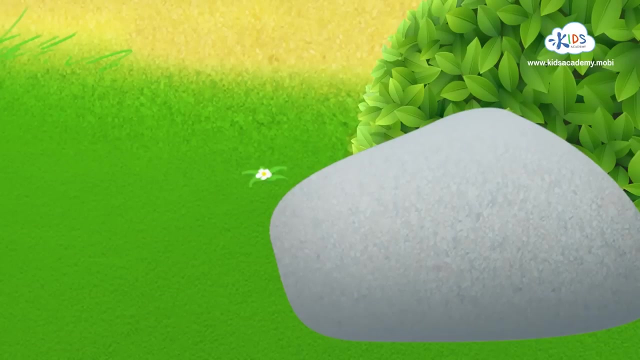 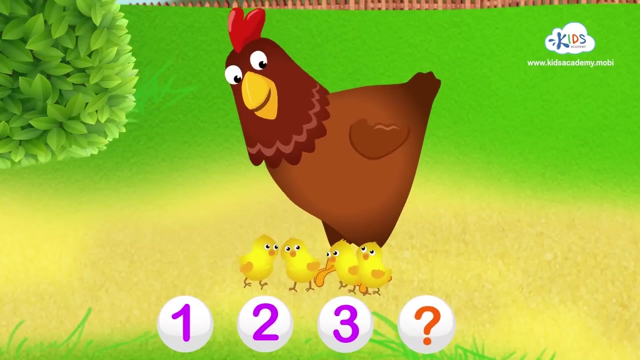 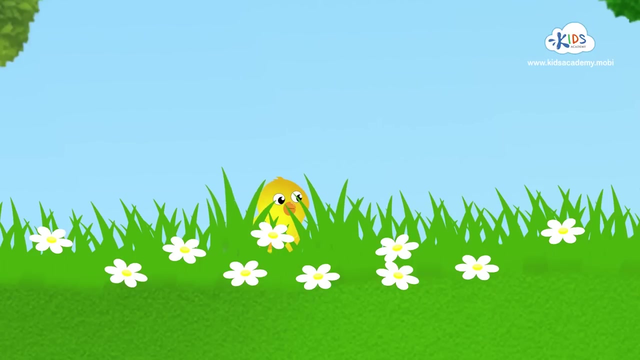 Two, Well done. And behind that far away tree we've got Three little chickens now. Great job. Let's go have a peek behind that big stone. That's Four, And the littlest chick is right in the flower bed. 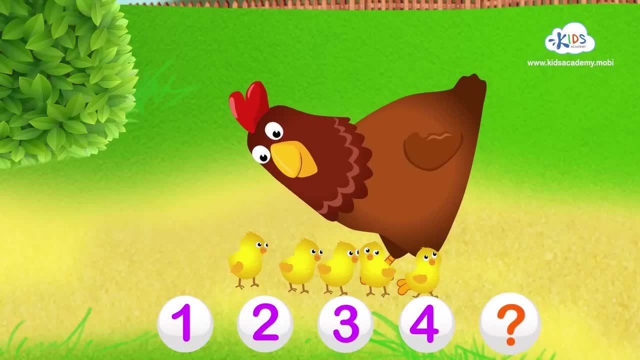 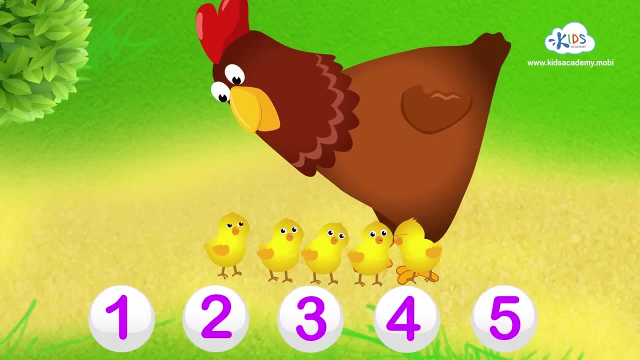 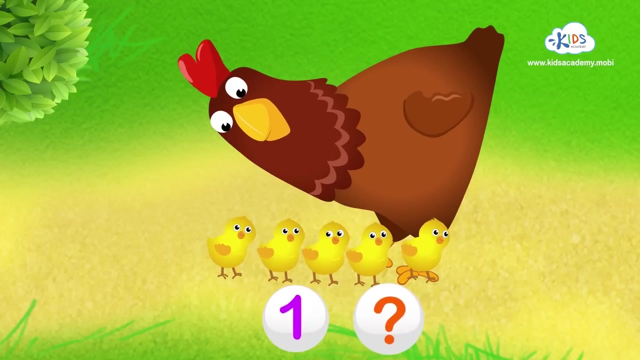 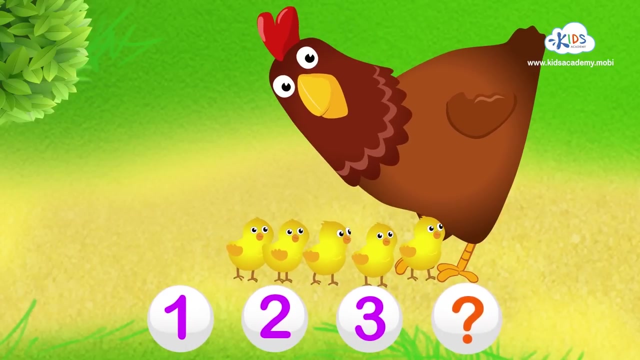 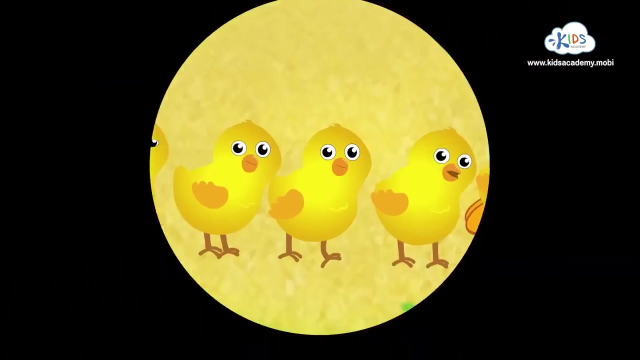 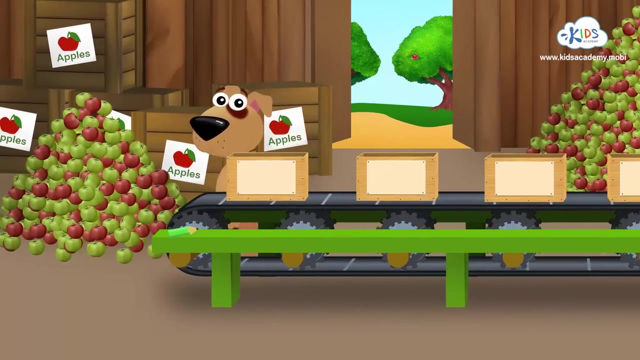 Great, That's Five little chicks all together. Let's count again and check Everybody. count with me: One, Two, Three, Four, Five. Great job, Bye, bye. Hi there I'm Toby. Can you see those sweet juicy apples? 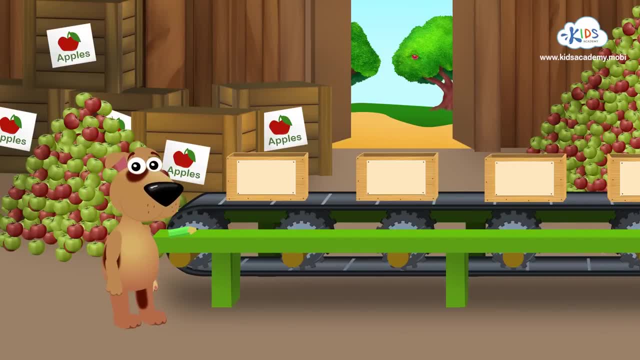 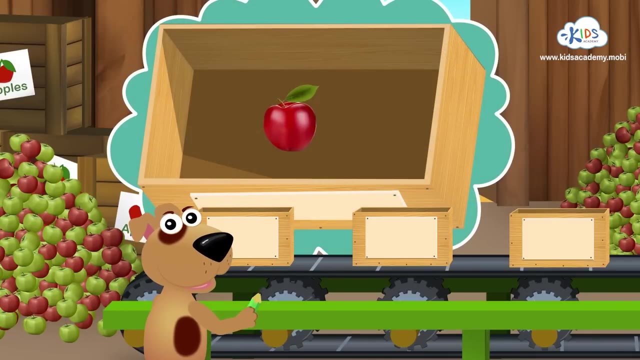 I'm going to count them and write the numbers on the boxes. Do you want to help me count the apples and write the numbers? Great, Now everybody count the apples and say the numbers. apples and say the numbers. There's one apple in this box? Great, Let's write the number. 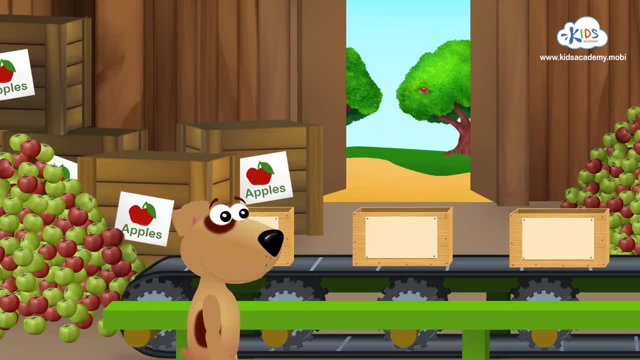 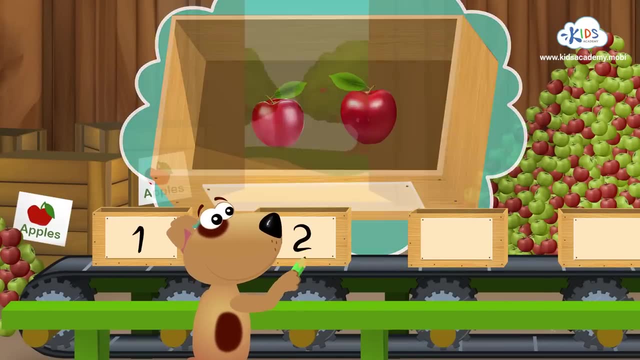 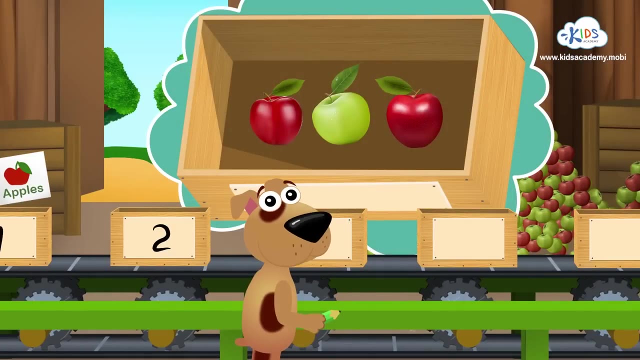 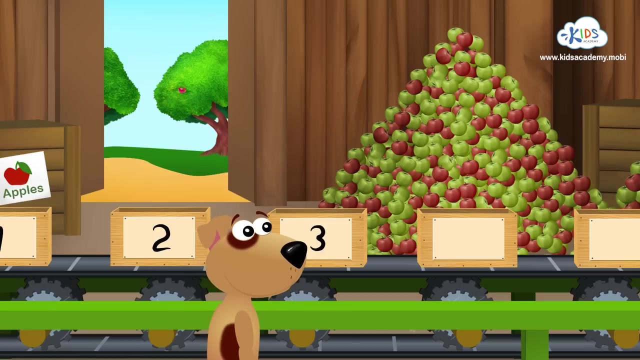 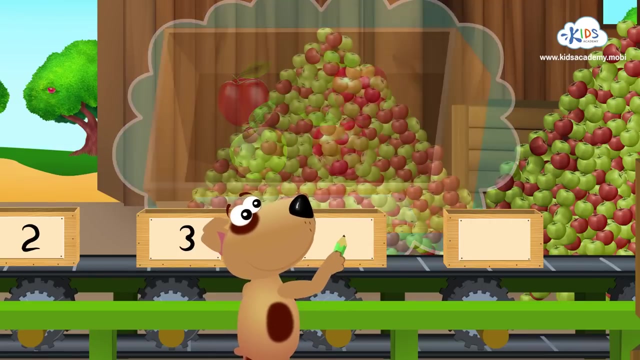 one here. Now count the apples in this box. We've got two apples here, Great. And here's the number two. There are three apples in this box. Good job, Let's write the number three. How many apples have we got here? Four, Great, You're really good at counting apples.